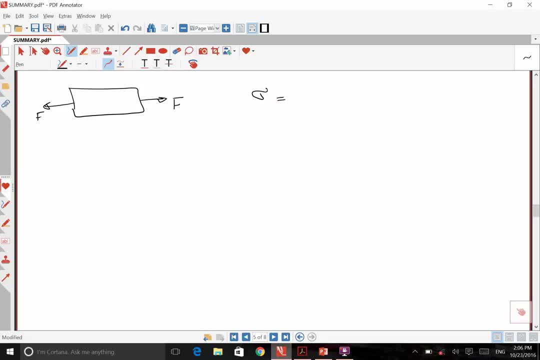 a stress for such a case can be defined as the amount of force over cross-sectional area. If I make a section here like section …. if I discuss a section here like section …. where exactly is that point like section … stress at this point, at section …. can 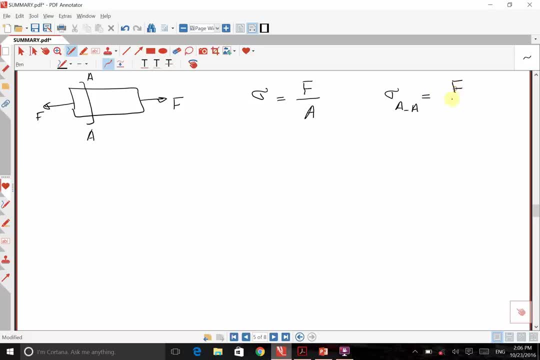 be represented as force over area. this stress here is average stress at a section. so by that I mean at section stress. here is a section at point, 자주 stress, which means that if this section is a section at point at a beside section, stress at this region is a like. this area apply to the point. if that's this position choice factor at that point. so, like here, a stress at a section here is running force and this is stress at point at section a. From this pie you can see that the stress here is coming from the action a. So by that 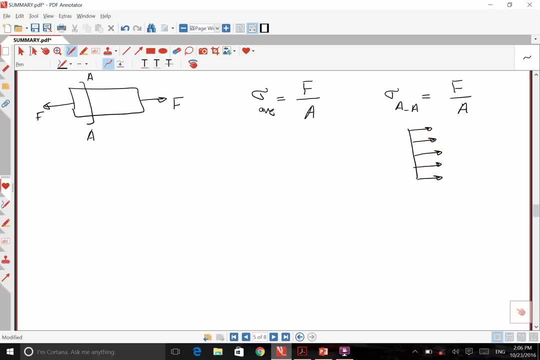 at all points at this section are assumed equal and equals to an. equal to F over a. if I had a hole here like that, if this section is far from a stress at this section can again be represented as this equation. but if that's so close to. 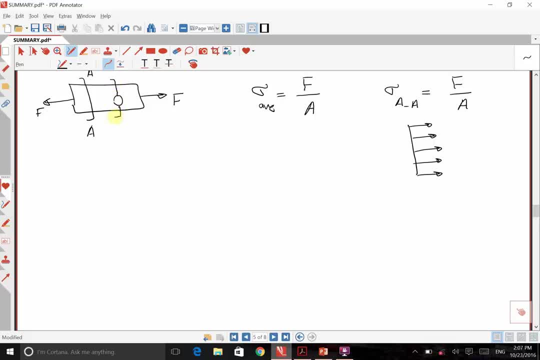 the hole and if it goes through the hole, like if I have a section like BB, a stress at section BB is not equals a stress as section a a. what important is for us in this chapter when we are talking about the stress, any type of stress- it's not a stress at each point- is: 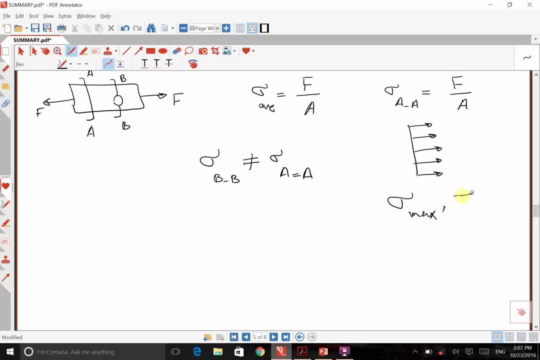 maximum stress. it doesn't matter if it's normal or shear. the maximum stress is important for us because we want to design something. and when you want to design something, the point that maximum stress happens at is important for us, and we want to know the maximum strength of the material. so if you want to find the 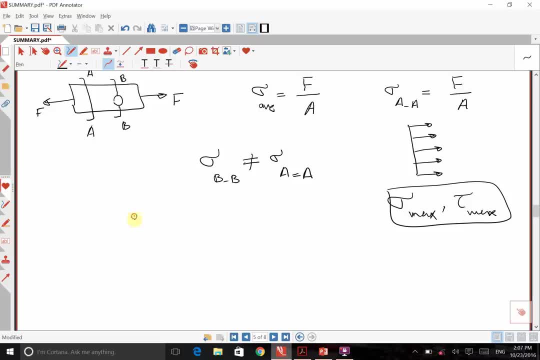 maximum stress. for this case we need to find a stress at around the hole where there is a stress concentration. so sigma. at section BB the maximum stress is again F over A, but we need to multiply that one by coefficient, which is KT. this means that we can just normally find a stress and after multiplying what that coefficient, 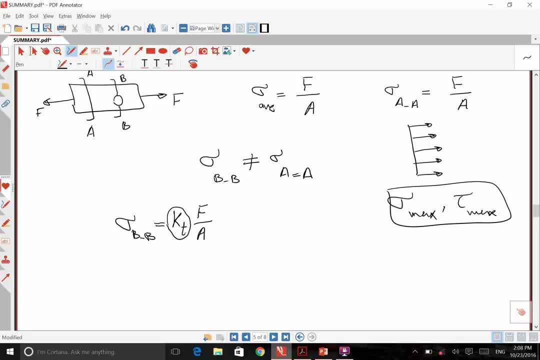 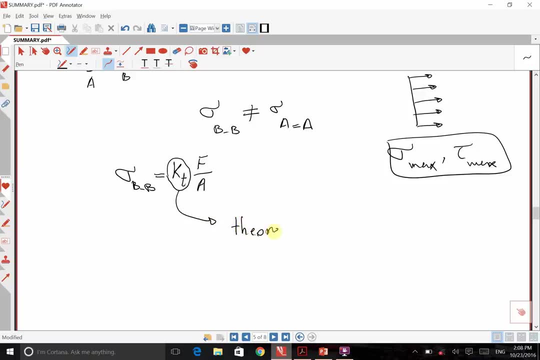 we're going to find the maximum stress around the whole. this KT is called theoretical stress concentration factor. okay, in order to find that KT, we need to go to a table that I'm going to refer to that one down the road. that's the first point that I wanted to mention. okay, the 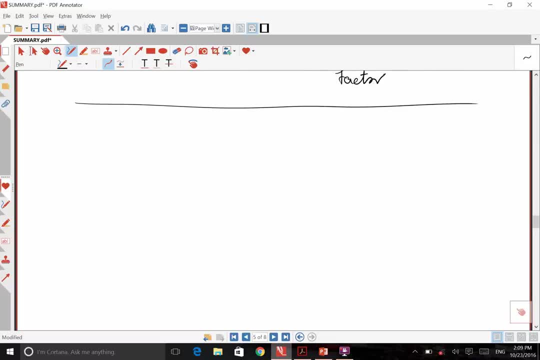 second point is about loads and stresses. we can have two type of stresses. okay, so we can have two types of stresses. so we can have two types of stresses: normal stress and shear stress. stress, by definition, is force over area, and we discussed about the difference between a stress and pressure. normal stress means: 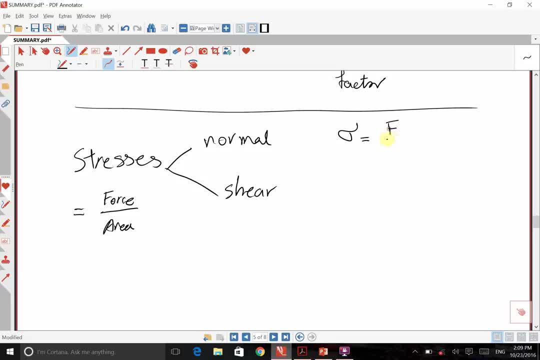 which we show with Sigma is when the load is axial or, yeah, when we lose axial. we can define that one and, for shear stress, that load is somehow not perpendicular to the cross section, is kind of parallel to the cross section and happening in the specimen, like that. okay, we don't have any problems at this point for loading. we. 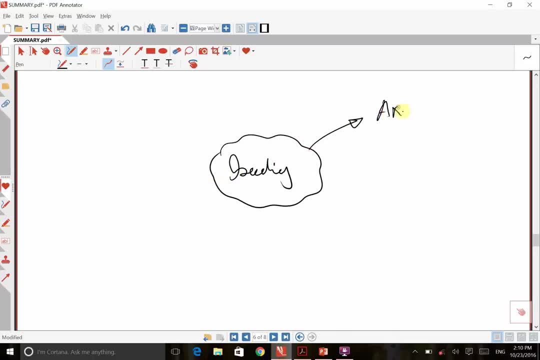 can have different type of loading. we can have axial loading. if that's our a specimen, this is axial loading F. this type of loading cause normal stress and the amount of stress is F over a. F is the amount of force and a is the cross-sectional area. so whenever at this chapter I'm saying a, 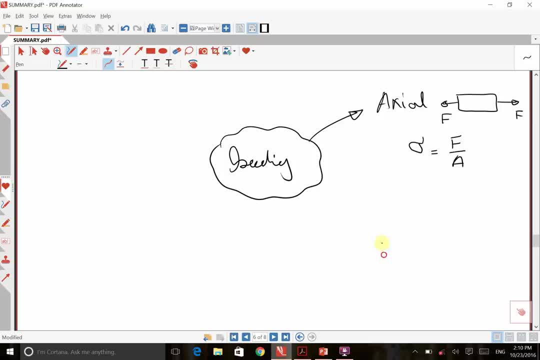 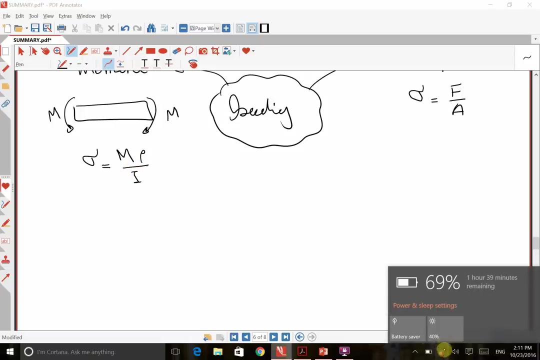 stress, I mean maximum stress. okay, so that's an agreement. another type of loading that we can have is bending moment, for example. I have specimen under this type of loading. I call this one M. a stress caused by this type of loading is again normal and can be written as M Rho over I, where I is second order. second moment of inertia. 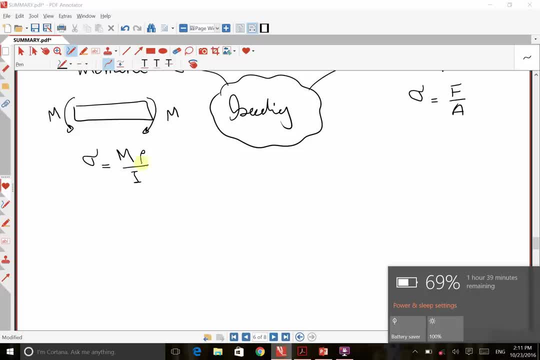 where I is, second order, second moment of inertia. okay, if I look at this cross, this, this specimen, from this side, if I look at this specimen, cross section, this row is a distance of a point that you want to read the stress from the center, for example. if this is the point that you. 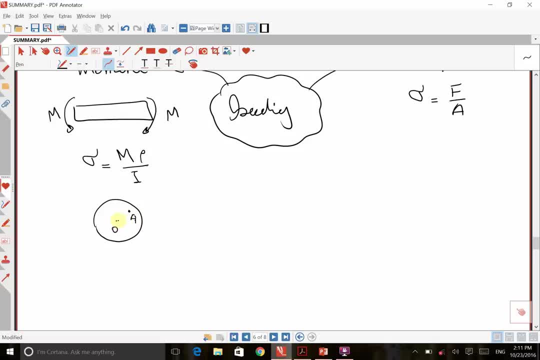 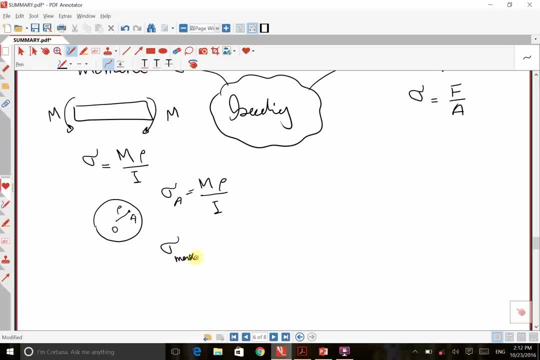 maximum stress. so what important maximum stress happens when I'm gonna say sigma max? happens when rho reaches to its maximum amount, which is radius. So maximum stress is M R over I. This is what's important for us. Okay, so this is a second type of loading. We can have third type of loading, which is torsion. 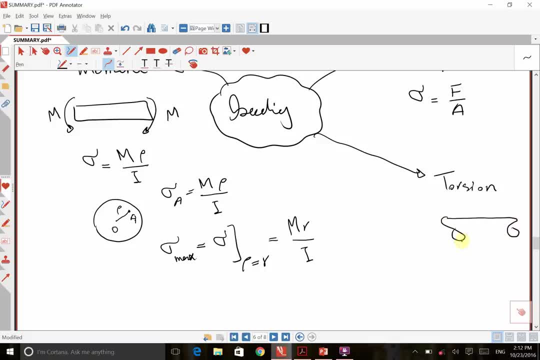 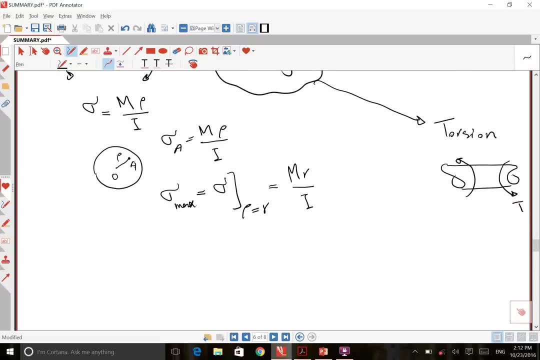 For example, I have a specimen like this and there is some torques like T twisting the specimen Here. I'm gonna have this and this. I'm gonna have a torsion here and I'm gonna have a torsion here. shear stress and the amount of stress will be T Rho over second polar moment. 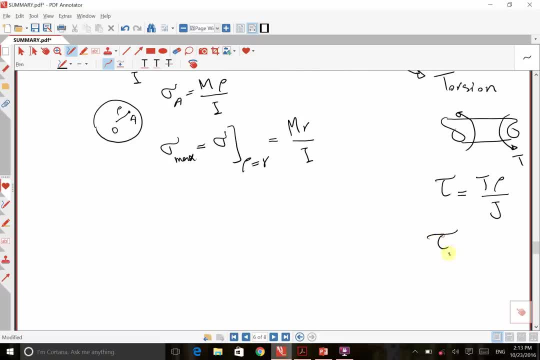 of inertia and the maximum stress, which is important for us, happens when Rho is maximum, so that will be Tc over J. we can have force type of loading, which is a shear force. for example, when you have a specimen like this and some force like V is acting, that force happens, some stress, let's say VQ over I, thickness and 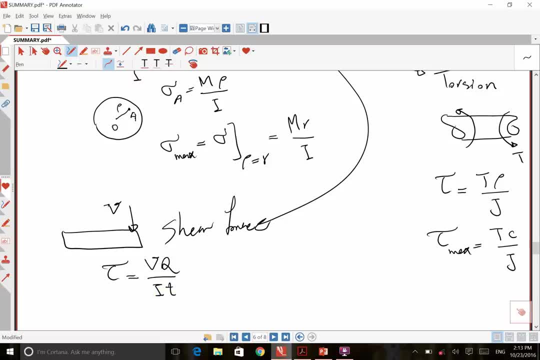 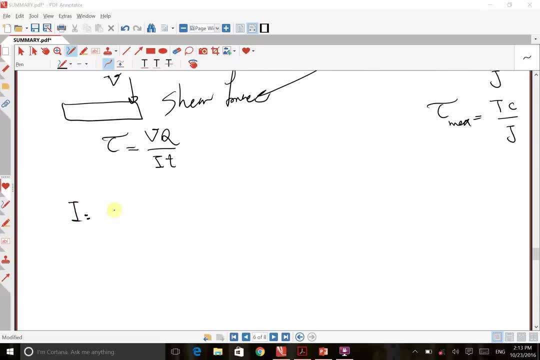 lobla. okay, if you wondered what this J and this I is, and I is second moment of inertia and J is second moment, sorry, second polar moment, our moment of inertia. these two can be found either online or at the appendix, section a 18, for example, for circular, cross-section I, for circular without any holes is P D to. 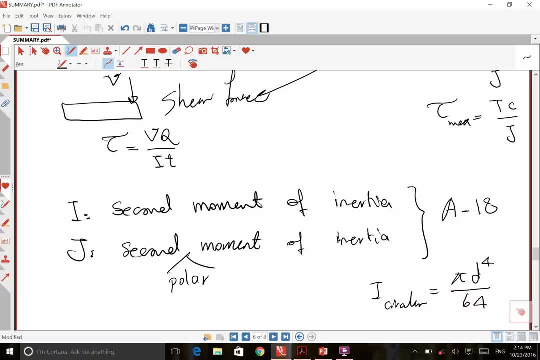 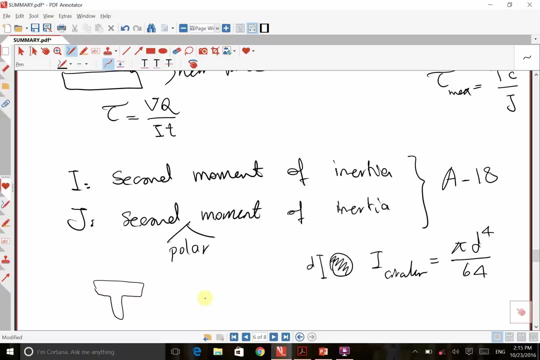 the power of 4 over 64, where D is the diameter of the cross-section. if that's like this- and this is the for the other type of cross-sectional, like for T being for rectangular one and the other types- you can go just to this table or you can find online. we don't have any problems. 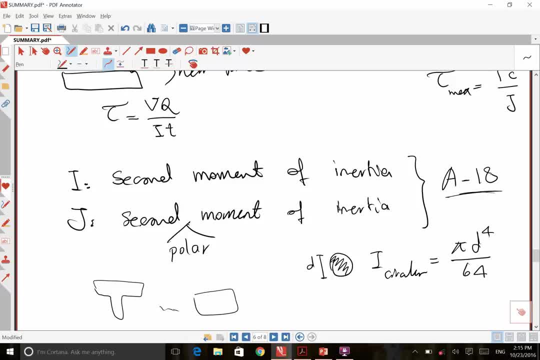 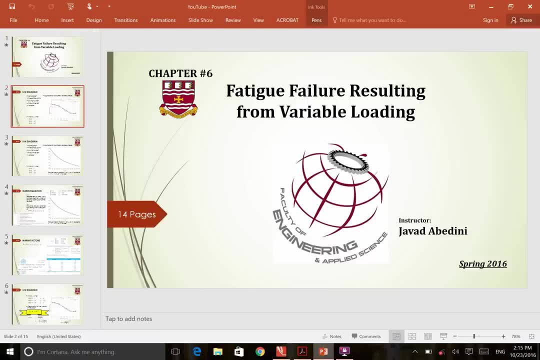 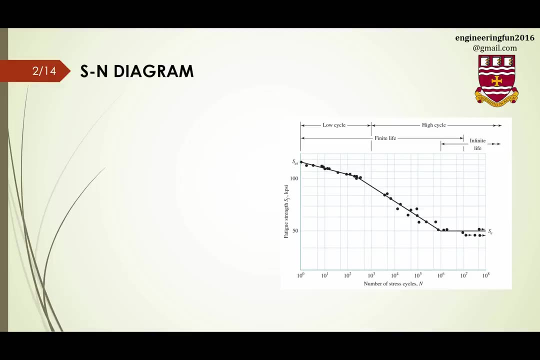 about this part. okay, now we can go to chapter 6 and see what this chapter is about. it's about fatigue failure resulting from variable loading. okay, so the first and important part of this chapter is about SN diagram. SN diagram is a log-log graph, so at the vertical axis we have 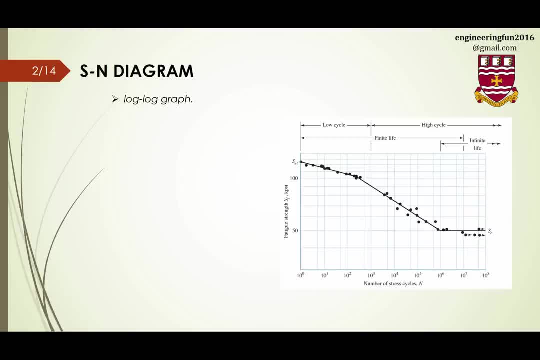 fatigue strength: SF- log of SF. and in the horizontal one we have number of stresses- log of N. okay, and this is valid for a completely reversed stress scenario. I'm going to talk about this one down the road. okay, there are three critical points at this graph. and this is the first critical point: when N is 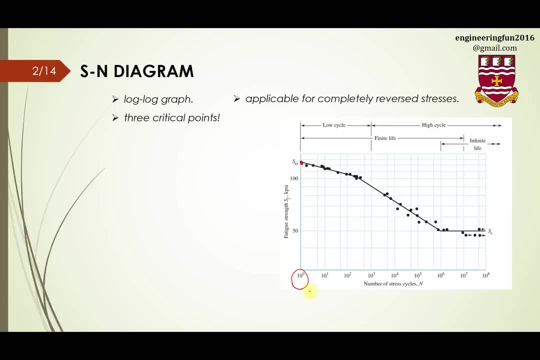 equals to 1. we said that that's a log-log diagram, so 10 to the power of 0 is 1. okay, that's the first important point. the second important point is somewhere here, when the cycle, number of cycles, or N, equals to 1,000. 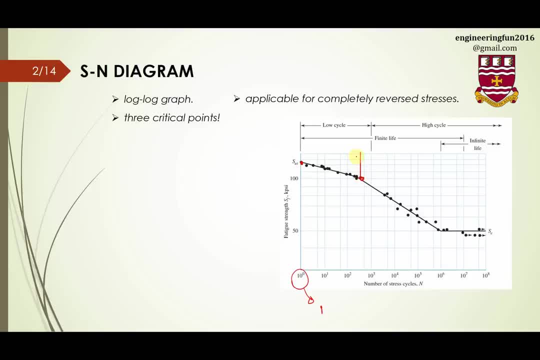 so I'm gonna say here, for example, I can delete this one, okay. and the third important point is about 1 million or 10 million cycles. these are three about and points for us, based on these important points. this graph can be categorized in different regions depending on the environment and development og health. 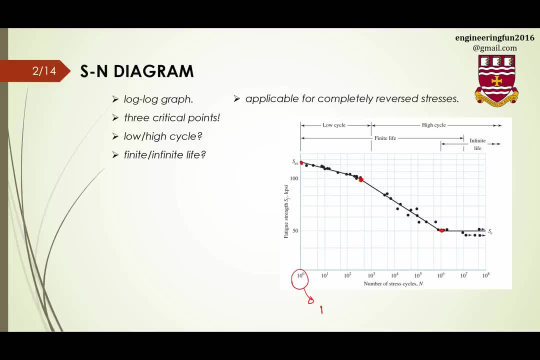 for example, whatever happens in the before the 1000 cycles is known as low cycle scenario here and whatever happens after them is high cycle, based on life, whatever before 1 million cycle is finite life and whatever after is is infinite life. for example, if I have a specimen like this: 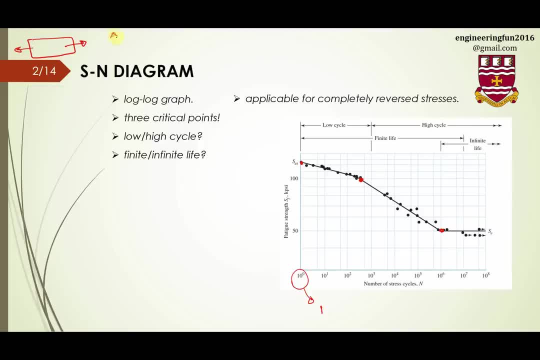 and if I put it under axial loading, this is what we recall from solids. if I want to draw stress strain diagram of this one, if that's a ductile material, it will be something like that. we have Sigma Y, yield strength here, ultimate strength here, Sigma UT and fracture stress and fracture. 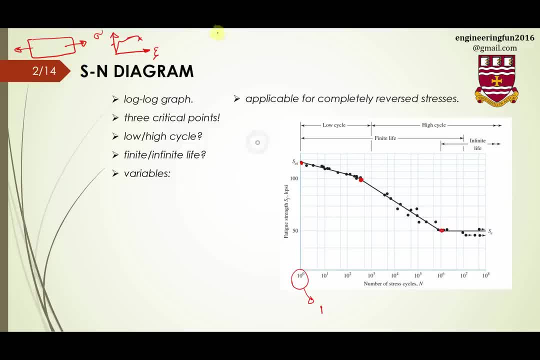 strength here. okay, stress you, if I want to draw load, I'm gonna say: if FT diagram for that one, that means that we are starting to putting load on the, on the material, until failure happens. so the amount of load is this much, is this much. so after one cycle failure happens. in this chapter we want to say that failure. 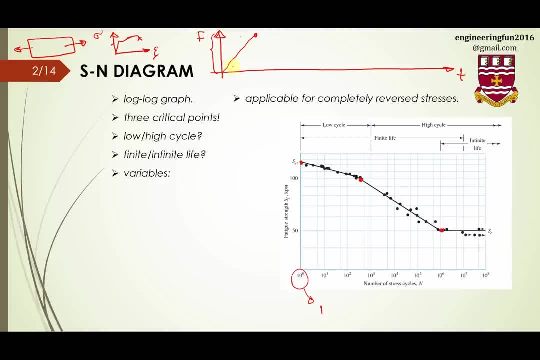 can happen with less amount of force. when we have a cyclic load, for example, we are increasing load like this, then we are decreasing load, then we are increasing load and then, okay, fracture happens here. so at this point the amount of force is less than our first scenario. so, with least, with 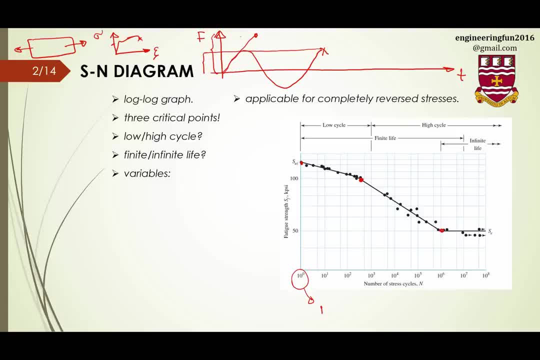 less amount of force, failure happens, and that's a result of cyclic loading. so we are somewhere here in this graph. sometimes we can have infinite number of cycles and failure never happens. this amount of force, which under that one failure won't happen, is represented a point here in 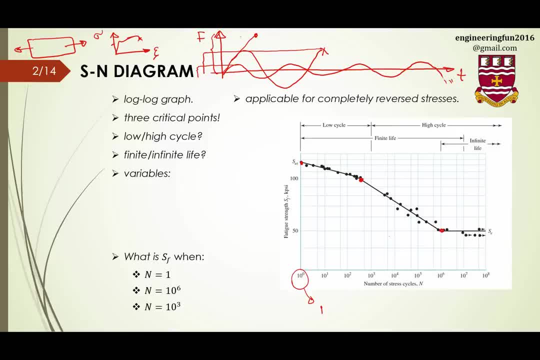 infinite life region. so for example, for this type of material, S F here is around 50. so I can say, if this amount, if this force is around 20 kpsi, I'm here and and we have an infinite life. so failure won't happen. there is one point here before I want. 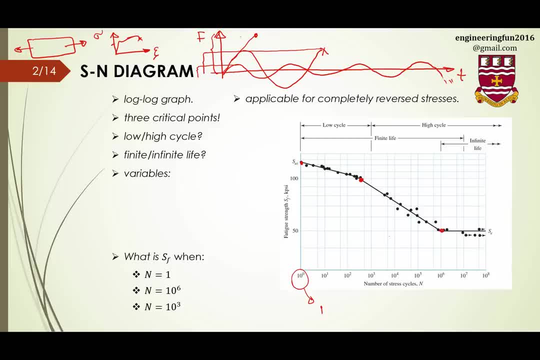 to continue, and that is about if we have- okay, I'm gonna tell that one later- the variables. one of the variables that we have here in the vertical axis is S F and oops is S F and that is fatigue strength index F in this chapter represent fatigue. the other 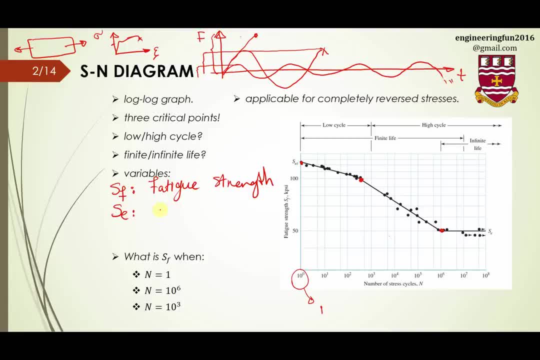 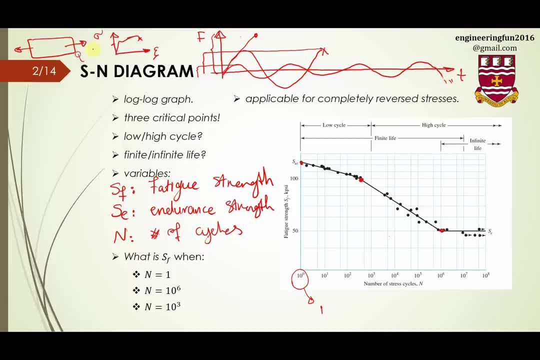 the number of cycles is 1.. That's for this case. here, For all these critical points, we know about the number of cycles. For example, for this one, this is 1, for this one, this is 1000, and for the last one is 1 million cycles. So we 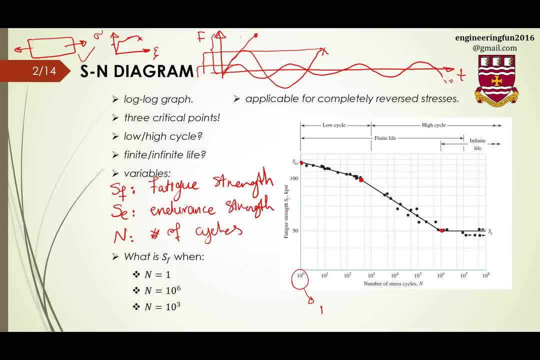 don't have any worries about the horizontal axis value, But for the vertical one, which is log of fatigue strength, we are worried and we need to know about these values here. For the first point, that's easy: SF fatigue strength is SUT, So that's this case. so we 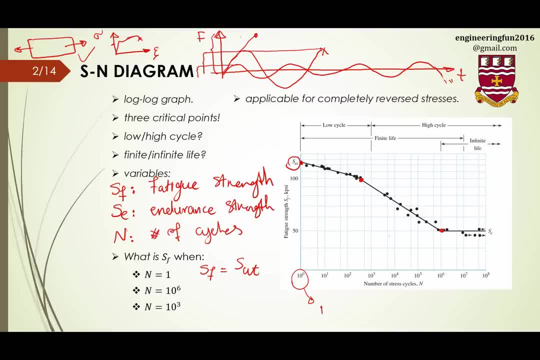 know that the failure happens at ultimate strength. For the last point here, this happens for each material at one point. this graph is not for all material, it's just for the specific type of material. but if I want to say general in general, this point is something that we called Sf. sorry Se. 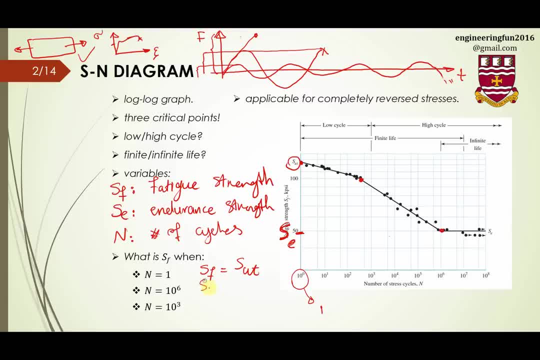 endurance strength. so Sf for 1 million cycle is equals to Se, and this is important for us. we know we want to know what is Se for each material, for each case, and we're gonna show you how to find Se. for this point, Sf is equals. 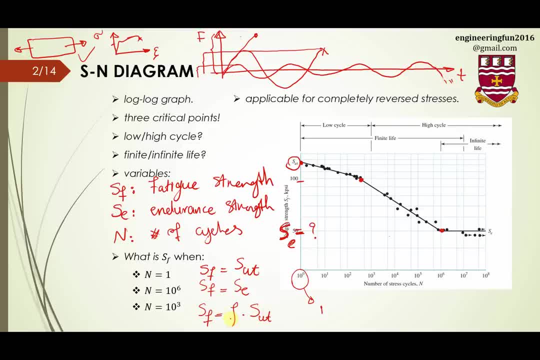 to some fracture of Sut. we can find this Sut from web- I'm gonna say online- or in some cases tables like table 820 in the Shigley's, or we don't have or it will be given to you. we don't have any problem for SUT. so once we found SUT we can find SF. 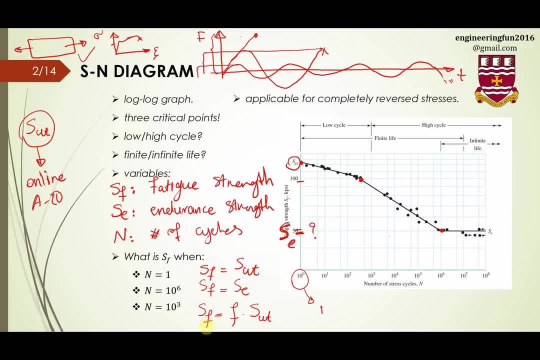 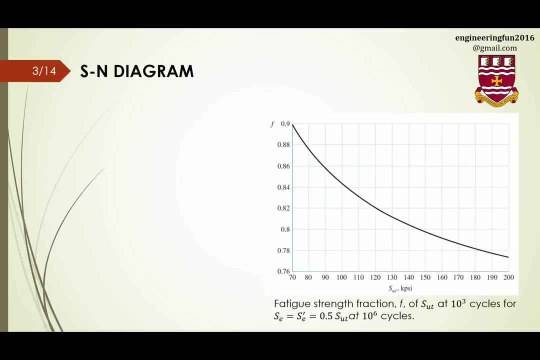 for the first point and in order to find SF for the second point, we need to know about this F. when you multiply F by this SUT, we're gonna find SF for the second point. okay, and this graph is used when you want to find that fraction. 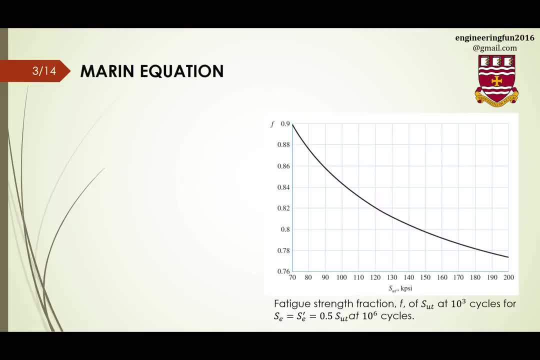 before I want to continue this graph. it shows that F based on SUT. for example, if in our studied case SUT is 170 kpsi, you're here, we're gonna go up find the intersect, then we're gonna go and read the number. so in this case, 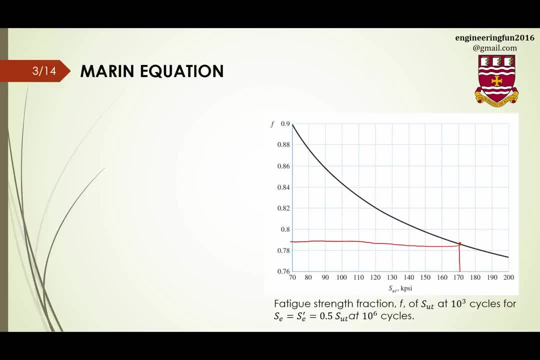 is ∙ına 79%. okay, if SUT is less than 70, so this line will continue like this horizontally. so, for example, if SUT is 50, I'm gonna represent and I'm gonna say this number as my F, and if that is more than 200, you can also make straight. 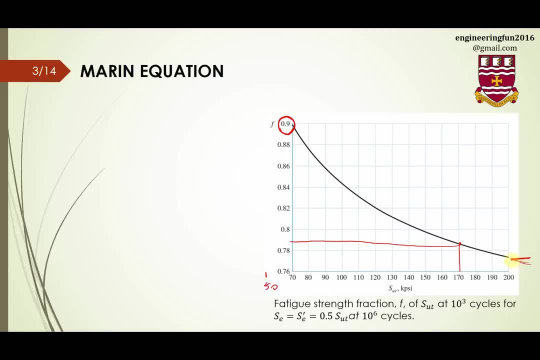 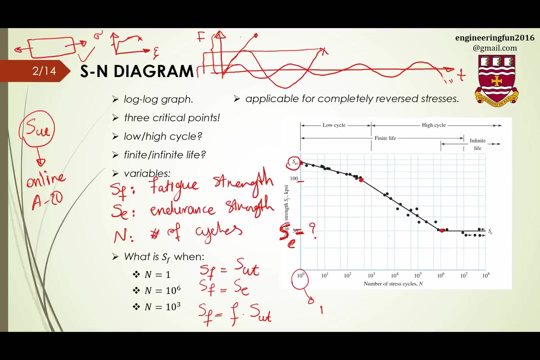 line, or you can interpolate something here and try to continue this one. it's not that important. for example, if SUT is 240, you can represent 77%, or, yeah, 77%, that's fine. okay, so we don't have any. if I come back to previous slide here: yeah, 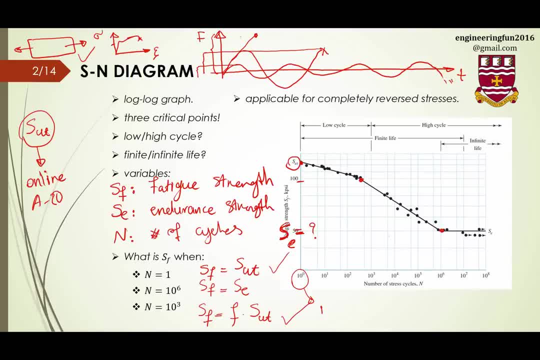 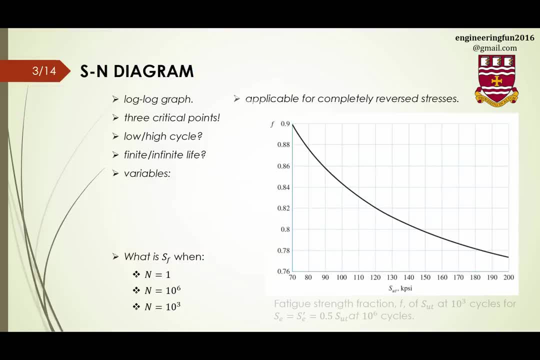 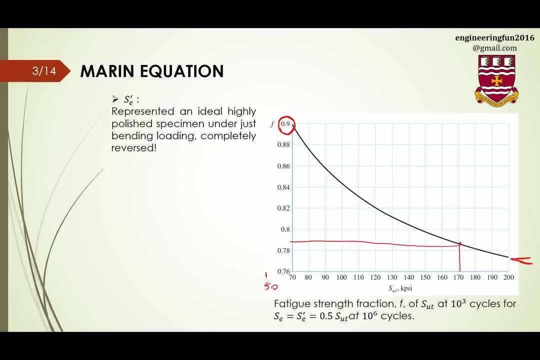 is SE prime. by prime we mean an ideal, highly polished specimen under just bending loading in completely reverse scenario here and this material can just be found under lab conditions. it's a very ideal scenario. when we know that SE prime, we can somehow find this SE based on that. 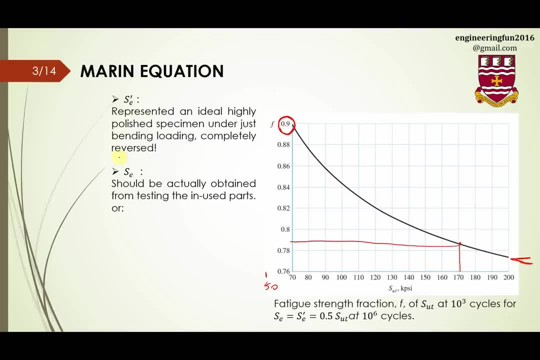 SE prime. the equation that relates SE to SE prime is called marine equation and this is a marine equation- SE prime times, couple of factors which ended up with finding SE in grand strength. actually, if you want to find SE, you need to take that part of machine and you need to 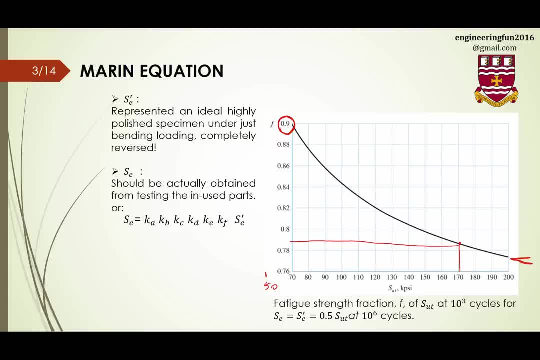 take it off and test it and find SE. but because it's sometimes it's very, very expensive to do that, sometimes it's not practical and you cannot do that. this is why we use these equations, when we put all these factors in order to find interest in endurance, stress, strength. okay. 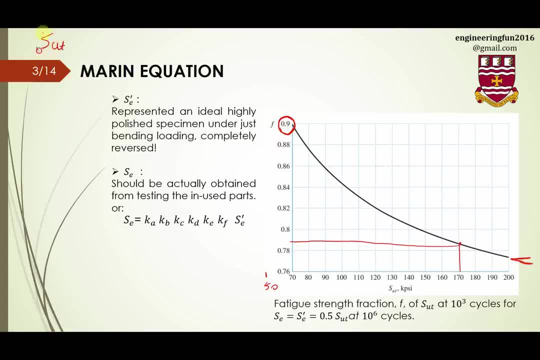 so so so far we know SUT and if we know SE prime we can find SE based on SE prime. here we want to know if there is any relationship between SUT and SE prime, because this is part can be found from internet and if you know this one we can. 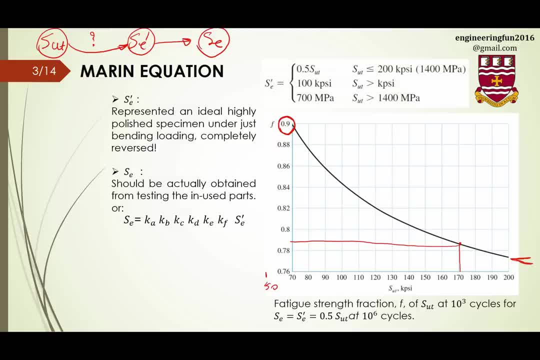 just put it here and find SE. this question mark can be answered here That Se' is very related to. well, I can say it's all related to Sut. If Sut is less than 200 kpsi, Se' is half of Sut. In 90% of cases you are in the first line. 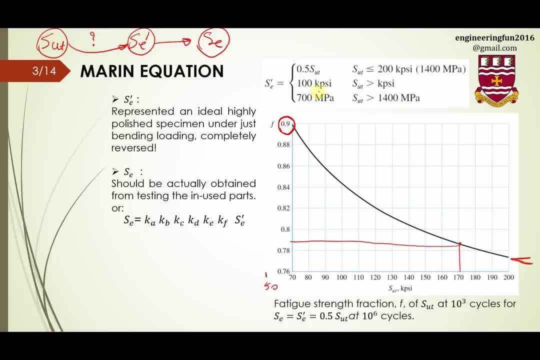 and 200 kpsi is almost 400 megapascal. If Sut is more than 200 kpsi, that's i. we are in the second line. so we can just say Se' is 100 kpsi And if Sut is more than, 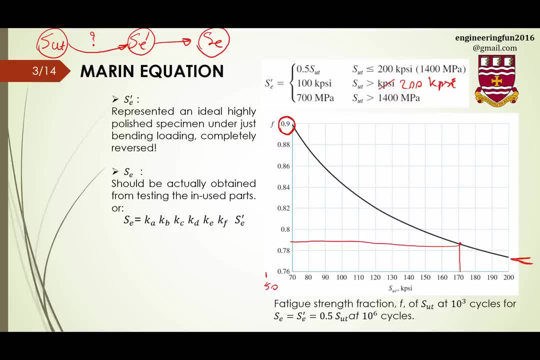 1400 megapascal. so if you're in the imperial system, we're going to represent this one for very high Se' Sut, And if we are in Si system, we're going to represent 700 megapascal as our. 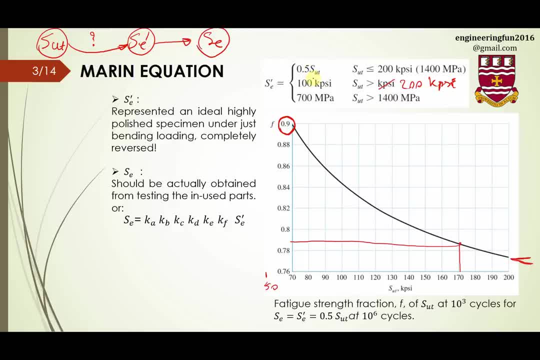 Se' So that means that we always divide by two. but for very, very high loads you don't divide that one by two, and you just divide the limitation by two. So if it's 200, here it's 100.. If it's 1400, here that's 700.. Okay, 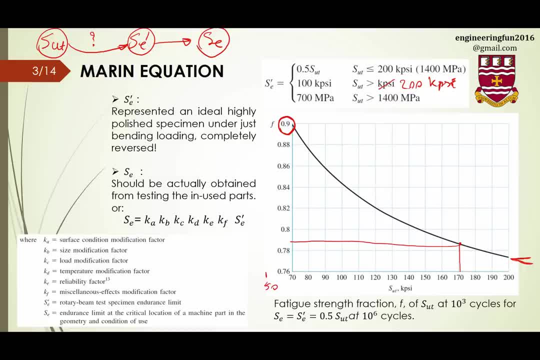 So we know about this Se' In order to find this Se' there are some factors: small k, i and that's not capital K. small k, Capital K is used for stress concentration and we're going to see in the future. Ka Ka is surface condition modification factor. 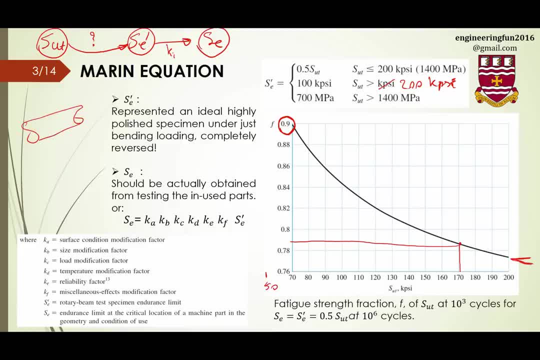 For example, if our real part has some scratches on the surface, we need to consider those scratches by applying this factor on our ideal specimen. Kb is size modification factor. It's used for size. Kc is load modification factor. Se' is for when. 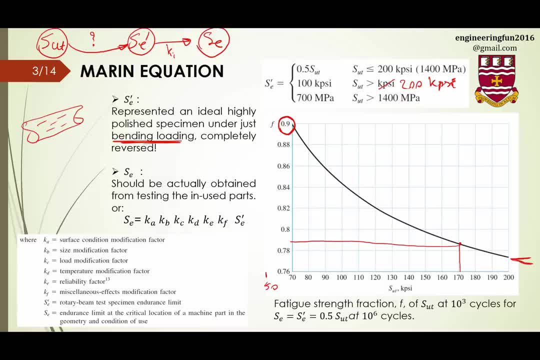 we just have a bending loading, But in reality we can have bending, we can have torsion, we can have axle, all type of loadings. If we have this case, what we need to do? we need to multiply the Se', which was for bending loading, by a factor. So after that, this means that we are: 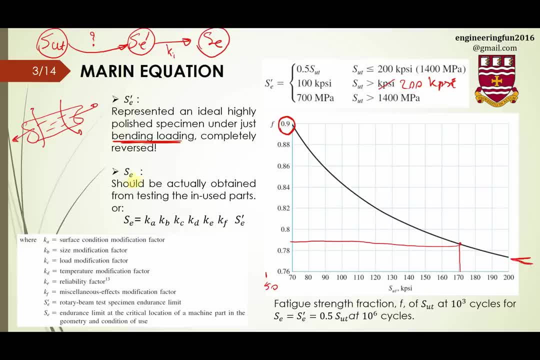 considering all type of loading. for our real part, Temperature modification factor, which is Kd, This is applied for very, very high temperature or sometimes for very, very low temperature. Reliability factor and miscellaneous effect modification factor- Usually that's one. We're not that worried about that one. Now I'm going to go and review all these. 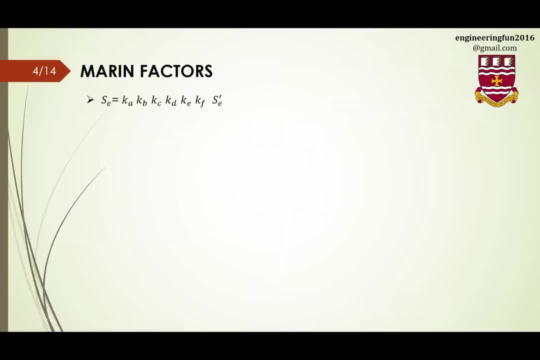 factors in detail, one by one. So that's marine factor. This is a marine equation, so we're going to talk about marine factors. The first factor is Ka, and that's A times SUTB. In this chapter it's very, very confusing. We have so many A's, so many B's. 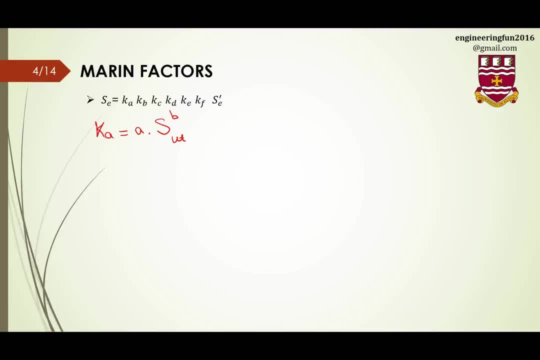 But anyways, we just keep the notation of the book. If you want to find Ka, you need to. we know SUT, you need to find Ka based on this equation: A times SUT to the power of B. This A and B can be found from this table. For example, if we are in imperial system, we are here. 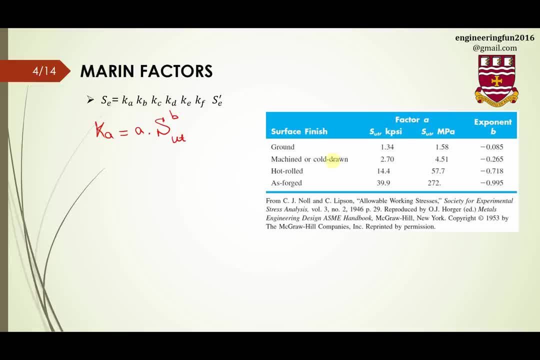 and if the type of surface finish is machined or cold drawn. so you are here. This factor A will be two hundred seven, two sorry 2.7, and the factor B exponent will be minus 0.265.. So in this case that would be 2.7. 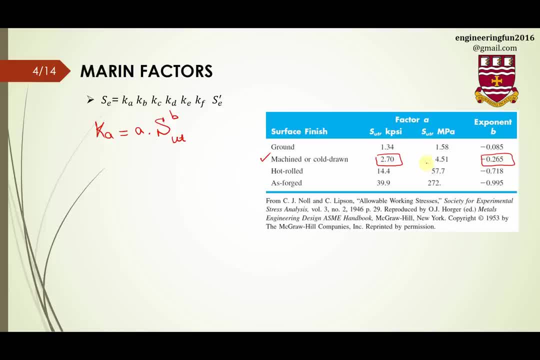 times SUT to the power of this number. And if you are in SI system, exponent B is the same, the coefficient here. we need to report that one. okay, so that's for the factor a. for factor b, let's me erase these ones. okay, and factor b. we said that if there is an axial loading, 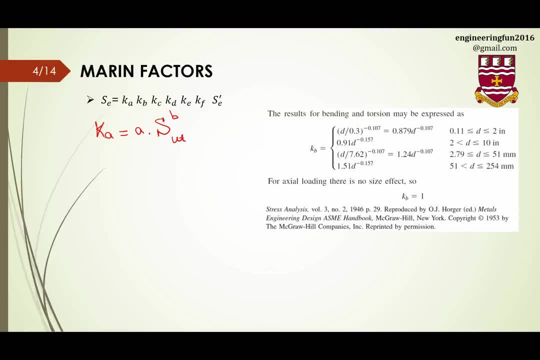 factor b is one, but if it's not axial loading, like if this is our specimen, like this, we have different type of and based on the diameter, say. if that's the diameter, kb can be reported by either of these equations, but the problem is the cross-section. 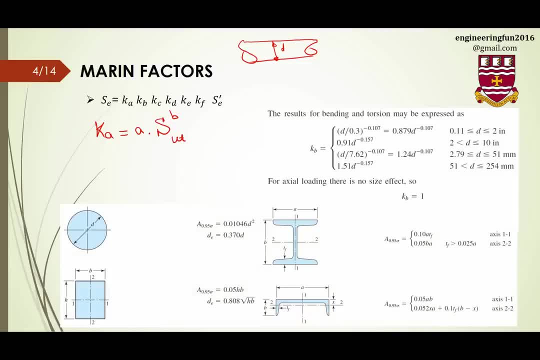 is not always circular. if it's not circular, if it's something like this, rather rectangular, or T or I or I being or any other shape, what we need to do, we need to here, instead of using D geometry, we need to use equivalence D, for example in this: 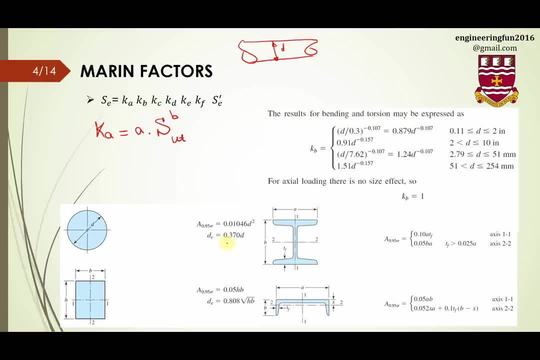 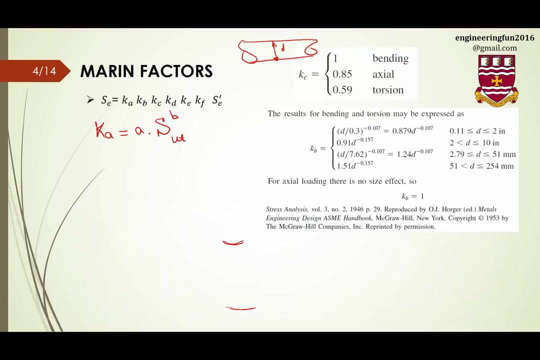 case: equivalence D. is this coefficient times real D? okay, if we have this case, we need to find the area a squared, find the square root and multiply by this one and use this equivalent e here. okay, KC, KC. it depends on type of loading. if you have bending loading, that's won. 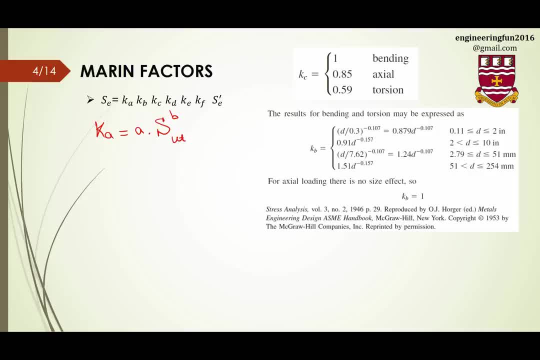 because sa prime is defined for pure bending loading. so by case fuckin R, you need to find the area of X squared and multiply that by this one, and that's what you need. If we have axial loading, we need to consider 85%, and if we have torsion, we need to consider 59%. 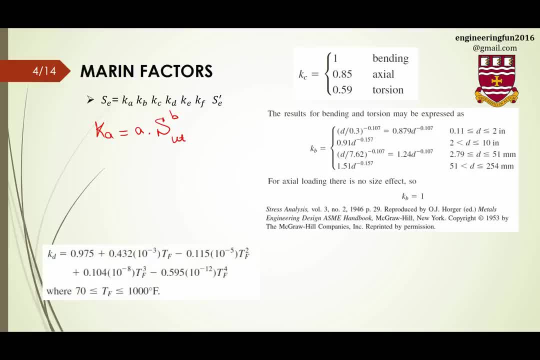 Kd again is temperature factor, so you just need to. that's for high temperature, when F is more than 70, and 70 Fahrenheit. that's important. The unit has to be in Fahrenheit. We're going to put that one here in Fahrenheit and we're going to find Kd and we're going to put it here. 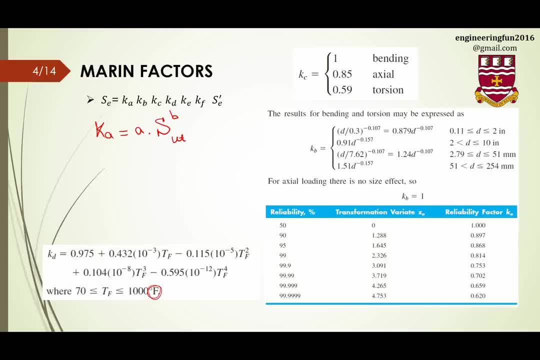 And Ke is reliability factor. It's interesting: when Ke is 1, that means that we have 50% reliability factor. So, for example, if you want to have 99% reliability factor, you need to put this number for your Ke. 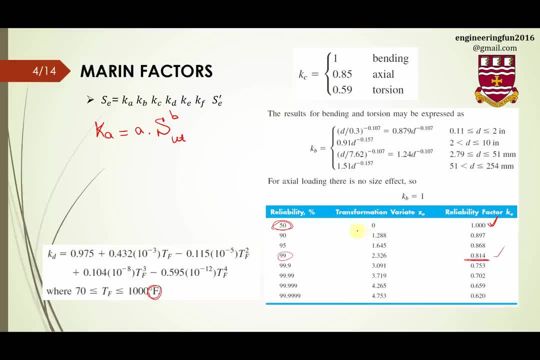 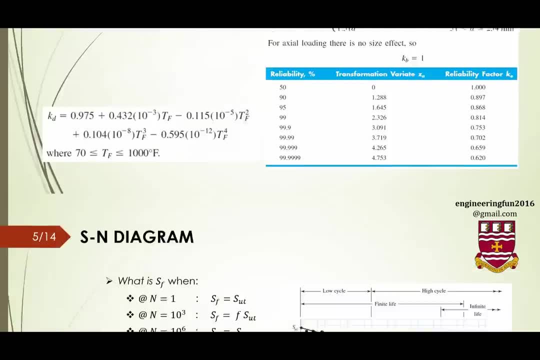 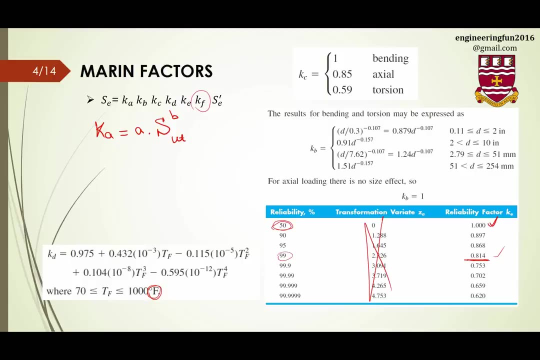 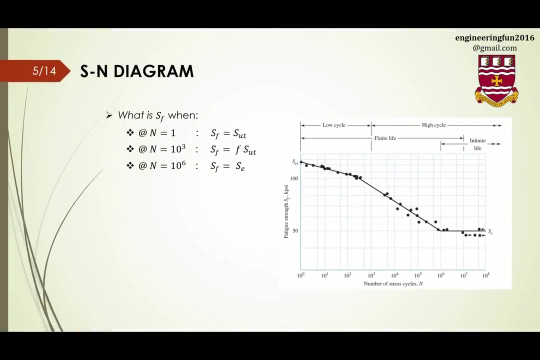 This Ke is found based on Za. You can just forget about this line and represent Ke directly. Okay, and this Kf is for other type of factors and it's usually 1.. Okay, we come back to Sn diagram. All this chapter is mainly basically based on this diagram. 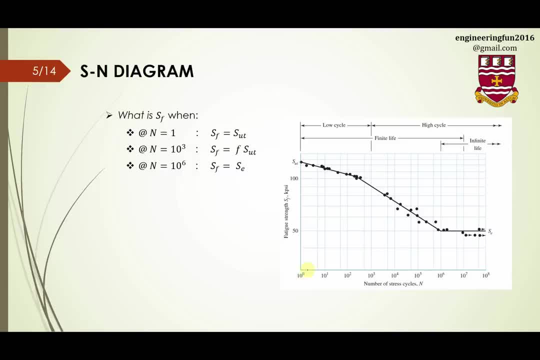 We said that for this for at n equals 1, for one cycle, Sf is Sut For 1000 cycles. For 1000 cycles, Sf is F times Sut, and for 1 million cycles, Sf is equals to indran's strength. 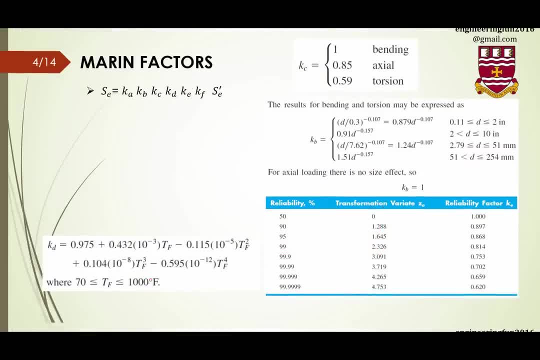 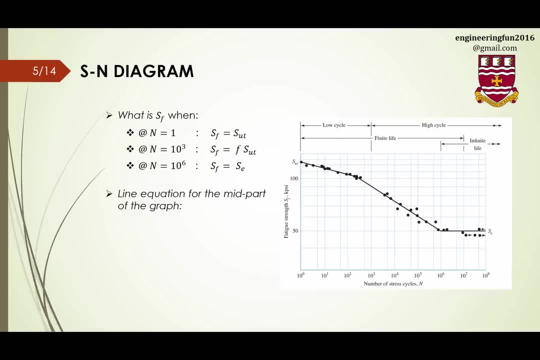 And we know how to find the indran's strength. sorry, Here we are curious to find the equation for the line at this area. here This equation, after doing some mathematics, can be represented like: Sf equals to A times Sut. 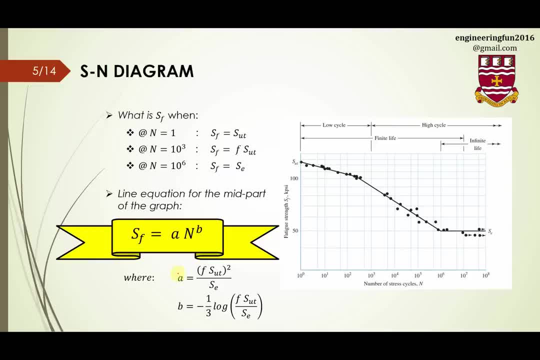 Sf equals to A times N to the power of B. Here this A and B is different from A and B in first modification factor. This A and B can be found based on ultimate strength and indran's strength of my material. Okay, this is a little confusing, but if you want, if you are asked to find the static strength for a specific type of, 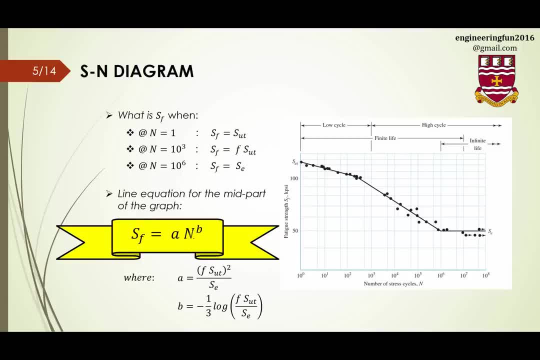 cycles. what you need to do, you need to put that number of cycles here and find these two factors based on SUT and SE, and then find SF for that specific number of cycles. Or there is another equation here, and this equation is when you have reversed. 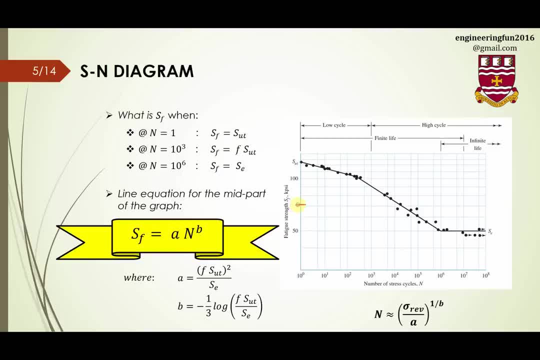 completely reversed stress, for example. if your complete reversed stress is something here you can continue to this point- find the intersect and read this number. you can find the number of cycles based on this equation here. This is this equation, but in different. 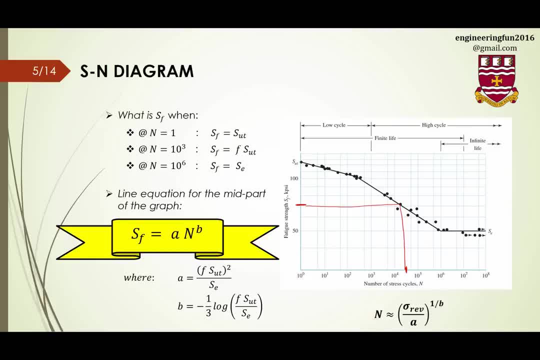 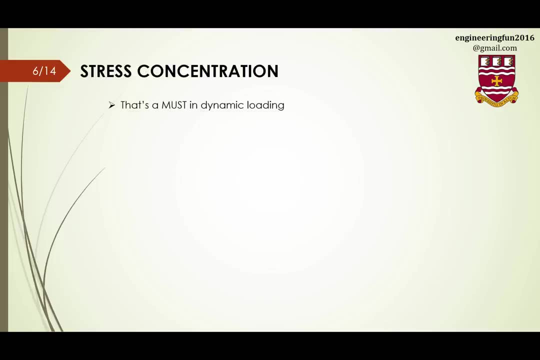 type of notation kind of. but whatever you can find here in these equations are not that accurate. they are all approximate, so that's why we have like approximation sign here. Okay, Stress concentration: Always when we have dynamic type of loading, stress concentration has to be considered. 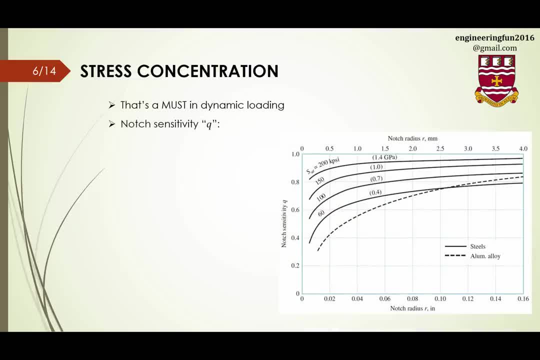 In order to. if you have static type of loading, stress concentration is just KT that we just talked about that before these slides. You can find it from the table. If you have dynamic type of loading, if you want to find stress concentration we need to find two factors: KT and Q. 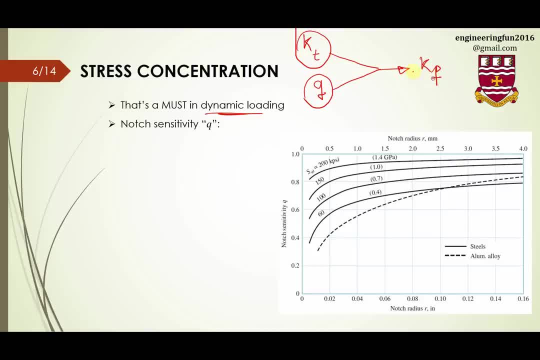 And combination of these two will give us some factors, which is called fatigue, stress, concentration. These two Ks are capital K, So we don't have any questions about finding KT. It's the same way as static type of loading. In order to find Q, which is not sensitivity, there are two ways. 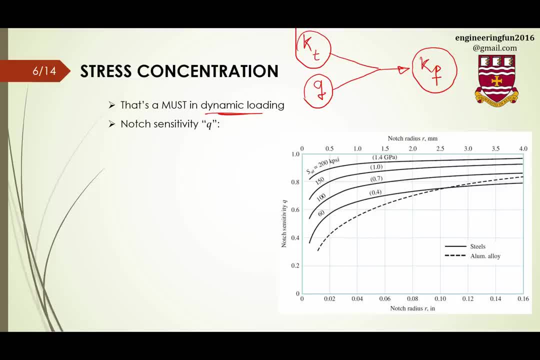 One way is finding Q based on the graphs. For example, if I have a specimen like this and there's a hole in it and there is axial loading, like that, if I want to find K, sorry Q for this material. I know about the radius of this notch here. 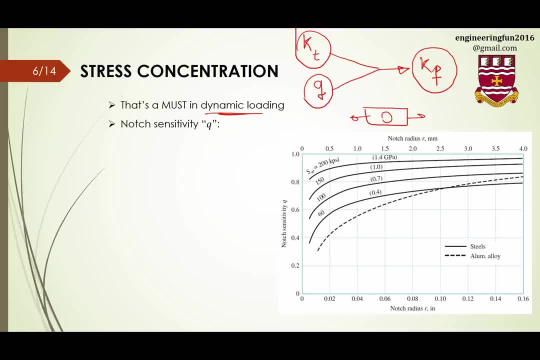 So what I'm going to do, based on the unit of the problem, if that's imperial, for example, for example, if the radius of that hole is 0.06 inches. I'm at this point, So I'm going to find, I'm going to draw a straight line. 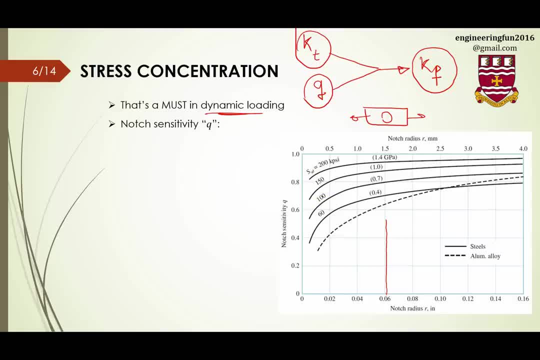 And if the SUT of material is, for example, 100 Kpsi, I'm going to find the intersect, which is this point. Then I'm going to read the number in the Y axis. So this is notch sensitivity, And for this case this is 80%. 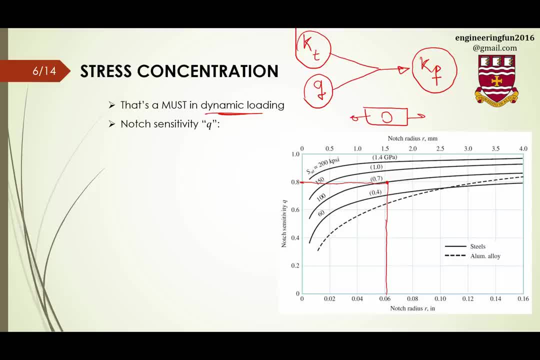 If I'm in SI unit, if the radius is, for example, 2.5 millimeter- So this is 2.5 millimeter, I'm going to start from top- And if the SUT of material is 1 gigapascal. 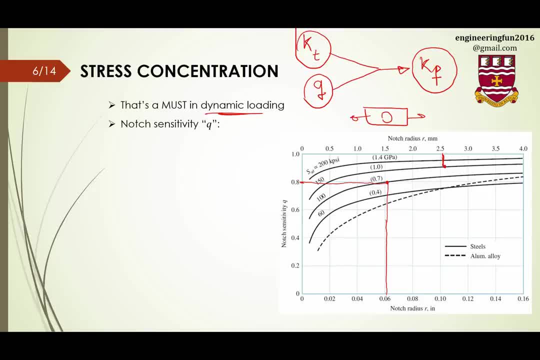 I'm going to find the intersect between the radius and that SUT And I'm going to read the number again in the left. So here, in this case that's almost 90%. So Q. one way to find Q is finding from the graph. 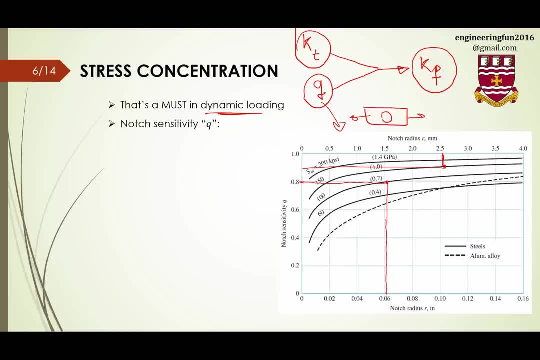 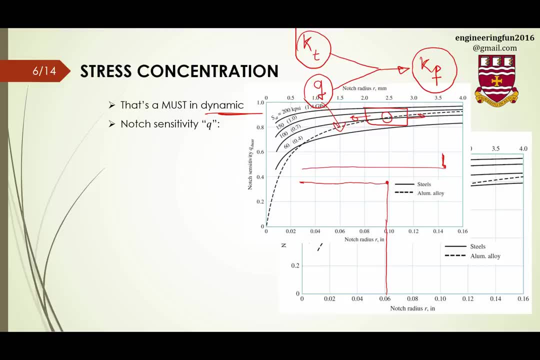 And this dash line is for aluminum alloys. Okay, This is like we use the solid lines, And there are two graphs for that one. One of them is for, like for axle loading that we discussed, And the other one is for shear. Okay, 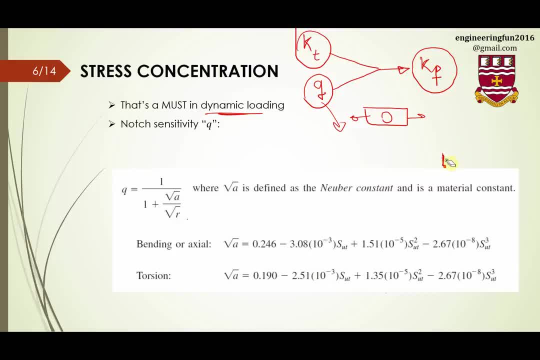 It depends on what type of loading that we have. We're going to use that. The second way to find Q: the first way was from graphs And the second way is from equations. Okay, Okay, So what can be found from this equation? 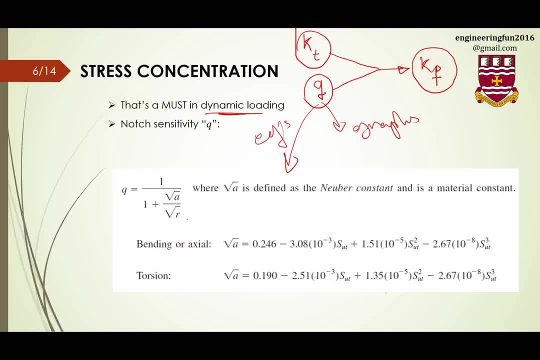 One over one, plus square root of A over R, We don't have any problems for the R. This is the notch radius. But what is square root of A? Square root of A is Nuber constant and is a material constant. It depends on the type of loading that we have. 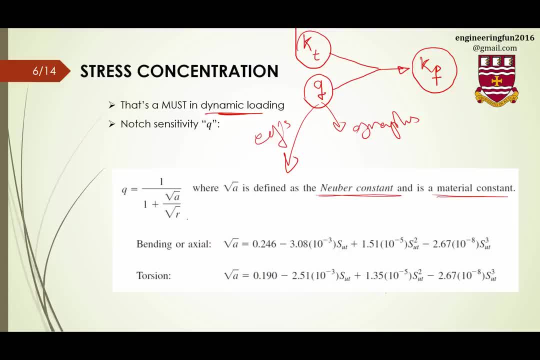 If we have bending on axial loading- in the first part we were using the first graph here- Square root of A can be found from this equation. So we know SUT, We substitute SUT here And we're going to find the square root of A based on this equation. 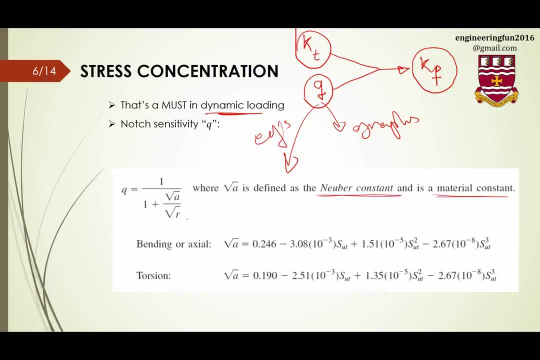 And if the type of loading is torsion, in the first part, we're going to use the second graph, Shear stress. Yes, Here we're going to find square root of A based on this equation. So square root of A is a function of SUT. 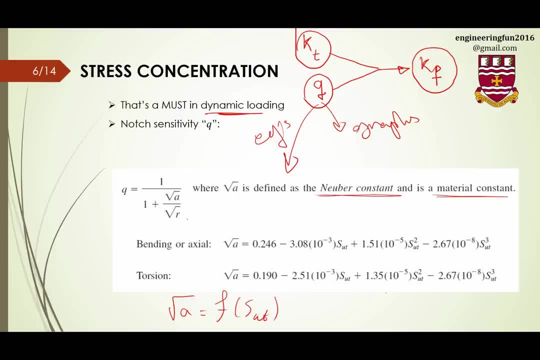 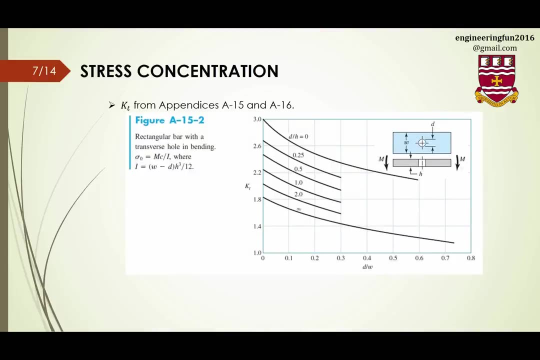 If I were you, I would always use the graphs, because that's easier and save lots of time. You just read the number here. You need to apply the number here and like, but that's up to you. Okay, I'm going to give an example here. 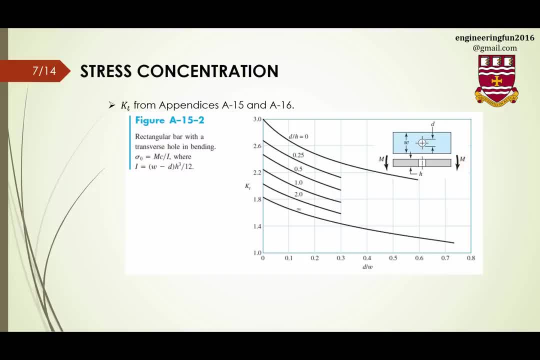 For example, if I have a specimen under bending moment. so I said I need KT and I need Q in order to find KF. This KT can be found from appendix A15 and A16.. For example, in this case, when you have a specimen under bending moment loading and the hole inside 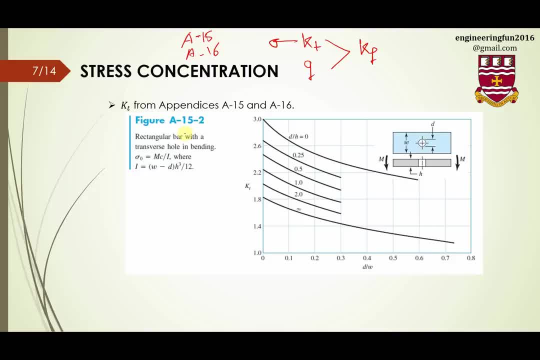 we need to go to this table here It's second number at this table- And we need to find the diameter of the hole over the width of the hole. For example, if you find that one and that ratio is 20%, 0.02,. 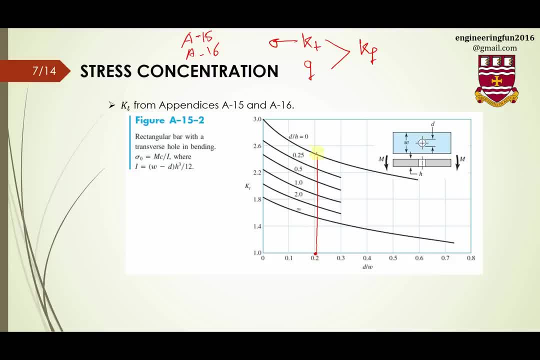 we need to draw a straight line, And this one is D over H, diameter of the hole, over the thickness or depth. So if that is, for example, one, if D is equals H, for example, we're going to report this number. 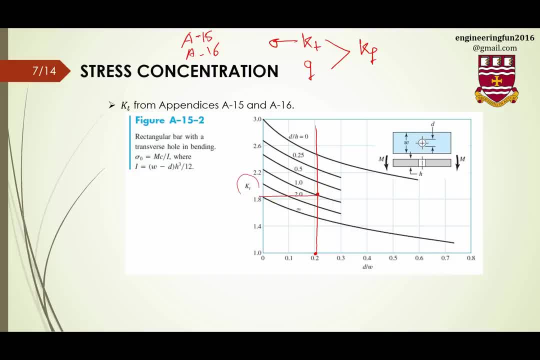 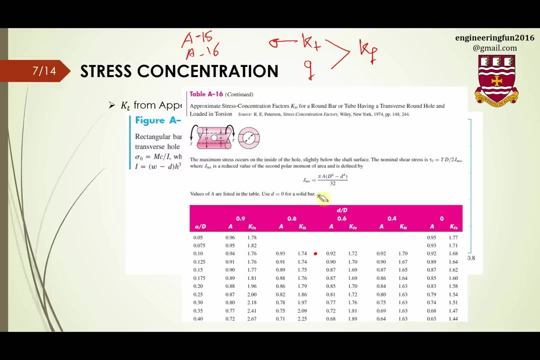 which is almost 185, as our KT theoretical stress concentration. We don't have any problems in that one. it's like solids And this is table A16.. In table A16, there are two tables: 16A, 16-2.. 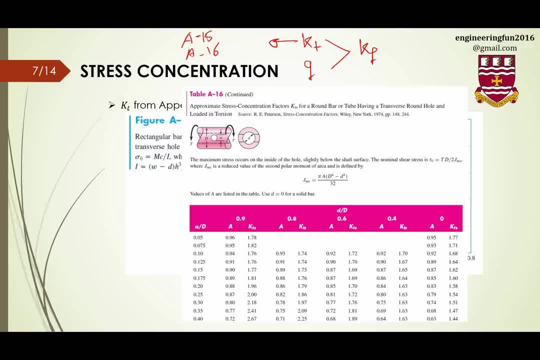 This is 16-2.. 16A is for bending, 16-2 is for torsion. For example, if you want to find stress concentration in this point, for this point you need to find J net, And this is PA over outer diameter to the power of 4. 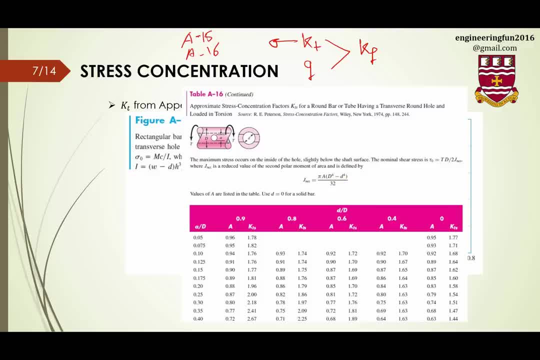 minus the inner one, to the power of 4 over 32.. D, capital, D and a small d are given in the question For finding A. what you need to do? you need to come to this table and based on A over D and D over D. 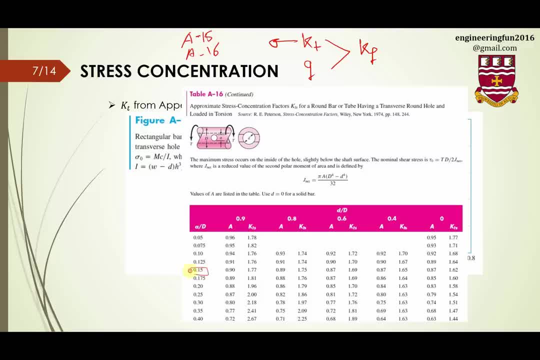 for example, if A over D is this much in your case and a small d over capital D, is that you need to present these two numbers? The first one is for your A, that here that you're going to use, And the second one is KTS for shear stress. 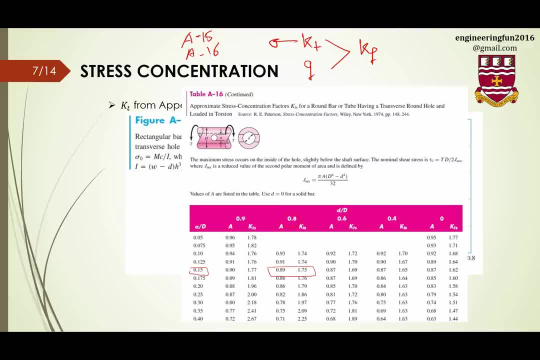 Okay. So when you want to, for example, when you want to find a shear at this point, the real shear, that will be KTS times, T knot. T knot is a normal one, So T knot here, as we discussed. 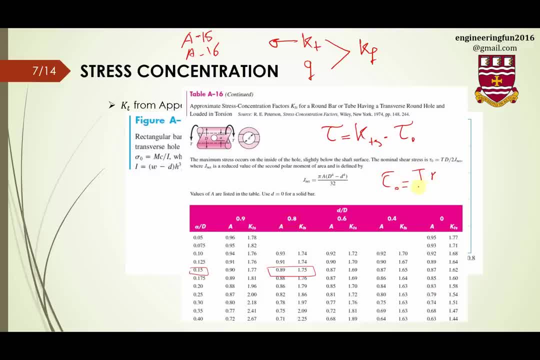 is TR over J- We'll talk about that in the before these slides- And I can say R is radius, So it's half of the diameter. I can say T- T over 2J- And this is exactly the equation that is shown in the table. 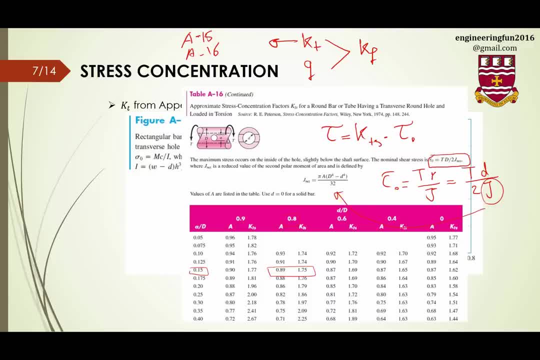 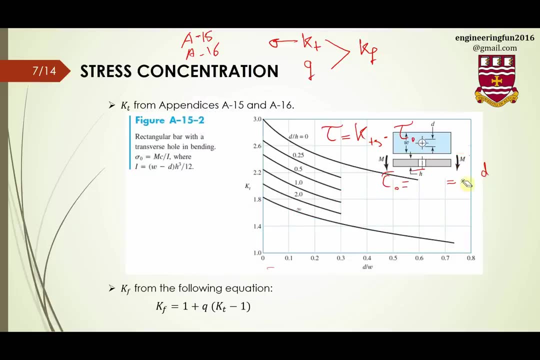 It's not that difficult And this J can be found from this equation. It's just reading a table. I don't want to spend that much time on these ones. We can figure out all the equations given the appendix. Okay, Once we get KT. 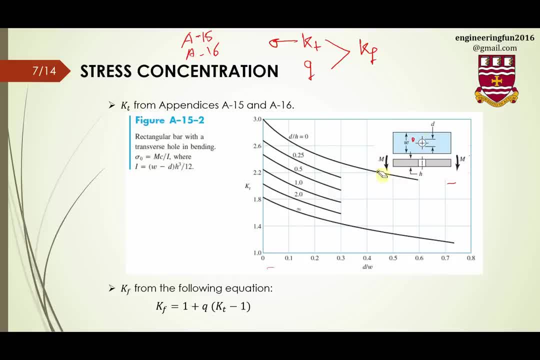 and once we find Q, we can find KF. based on this equation, KF is equals to 1 plus Q times KT minus 1.. Okay, That's an important equation for us. So KT can be found from these tables, Q from other type of tables. 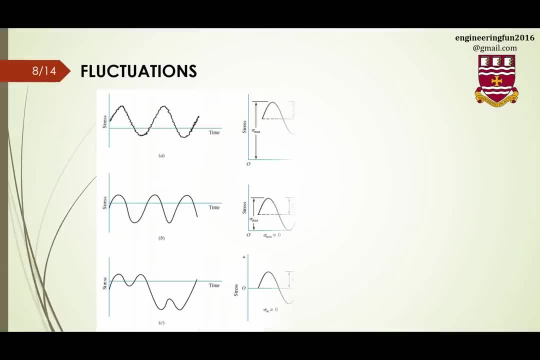 and we're done Okay. The last part of this chapter is about fluctuations. At the beginning of this chapter, when we said that SN diagram is for fully or completely reverse scenario, we mean this case Here: stress time behavior is something like that. 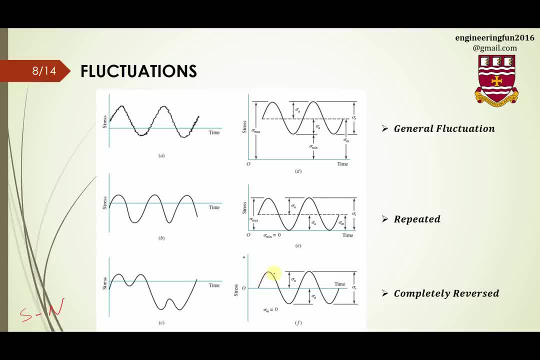 You start from zero, You go to some amount of maximum stress- I'm going to say tension- Then we go to compression, Then again tension, Then compression, And we hit the maximum amount of each one. Tension and compression, like that. 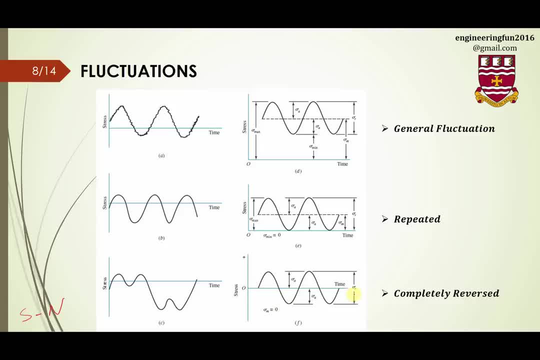 And we are fluctuating around time axis. This is called and known as completely reverse scenario, But in real part we don't always have this scenario. We can have repeated scenario. By repeated, it means that we start from something and we go to fully tension scenario. 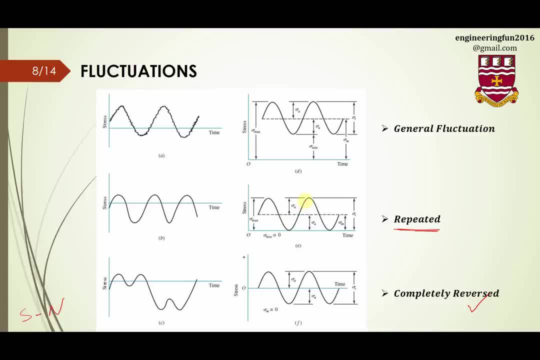 Then we go to zero. Then again we go to some amount of maximum, Then we go to zero. For example, if I have a specimen like this and I put bending moment on that, I can have this one as my maximum. 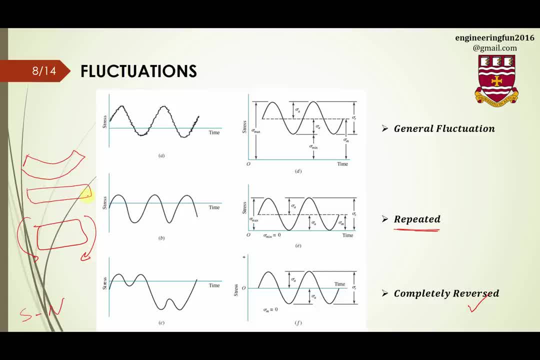 Then again make it straight. Then again, go to this one, Make it straight. Go to this one, Make it straight. So I don't go to the other section, I'm just looking at one side, for example, at this point. 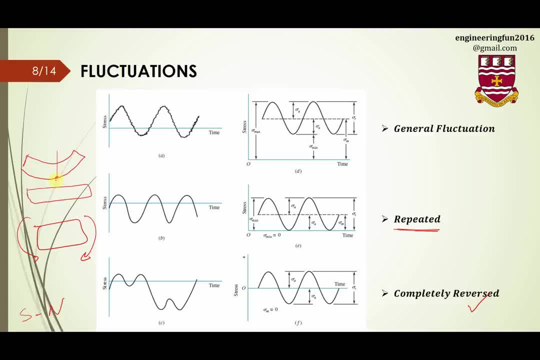 So this point goes to maximum tension because it's stretched again to zero tension zero. So that's repeated case And we can have a general fluctuation types. We can have some offset from time axis And we can fluctuating around something. 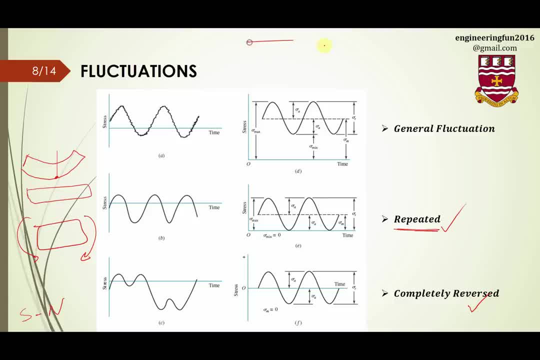 We can increase and decrease load. Okay, For example, we have a specimen like this And there are forces acting all over the specimen, And this force can be varied from 8 kpsi to 68 kpsi And both are in tension. 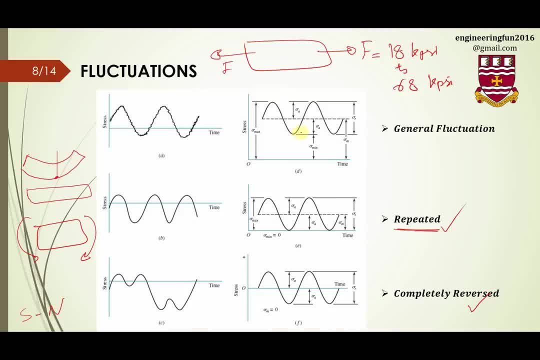 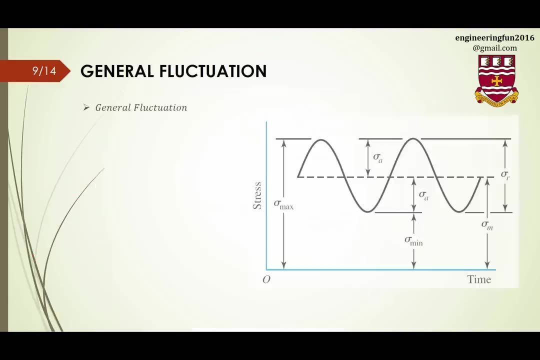 So that means we are here, 18, we can go to 68,, go to 18,, go to 68,, go to 18.. So the force is fluctuating and we are not around zero. Okay, This is what we want to study on now. 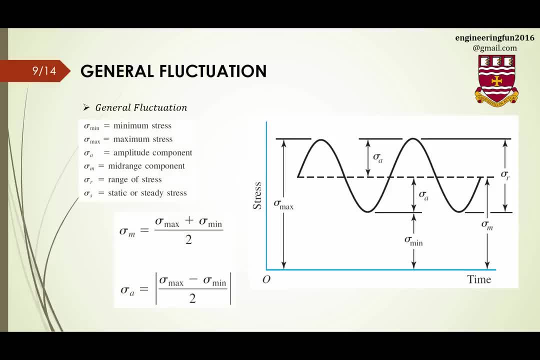 In general fluctuation scenario, there are two parameters that are important for us. The first one is the amount of offset, which is known as mid-range stress or average stress, which is maximum plus minimum stress divided by two. This is maximum minimum divided by two. 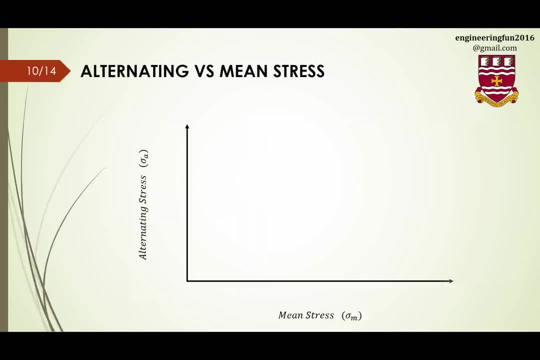 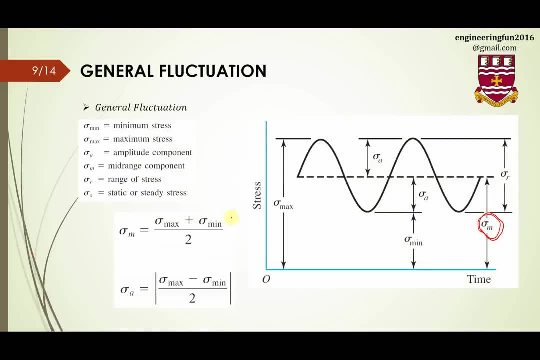 In our case, for 68, what was the other one? And 68 and 18.. So what we need to do, we need to those were forces. We need to find the stresses by dividing them by surface area And we just 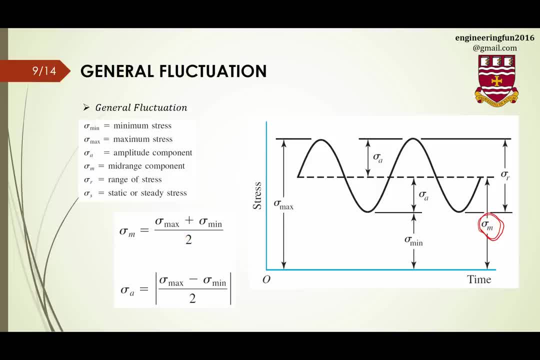 find the average. So this is the average one. Okay, The second one is the amplitude of this oscillation, which can be found from absolute value of differences between maximum and minimum stresses divided by two. So these two parameters, mid-range stress or average stress. 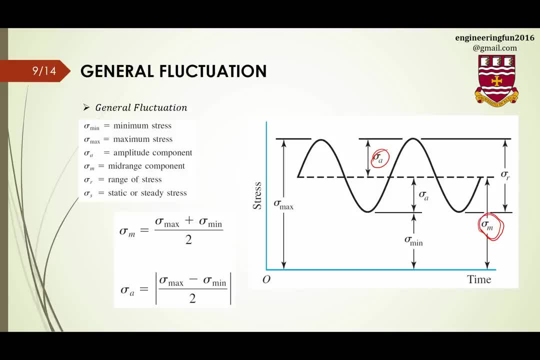 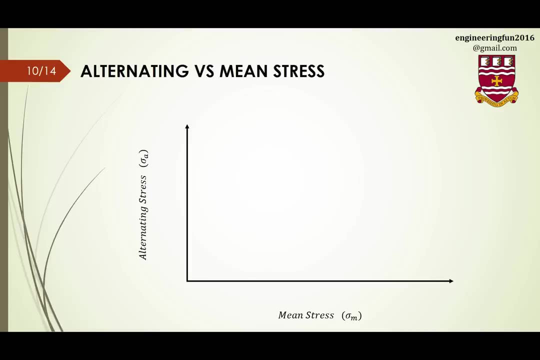 and alternating stress or the amplitude of this fluctuating, are important for us And we can get them based on these equations. Once we get these two equations, we need to plot alternating stress versus mean stress or mid-range stress. There are a couple of important points for us. 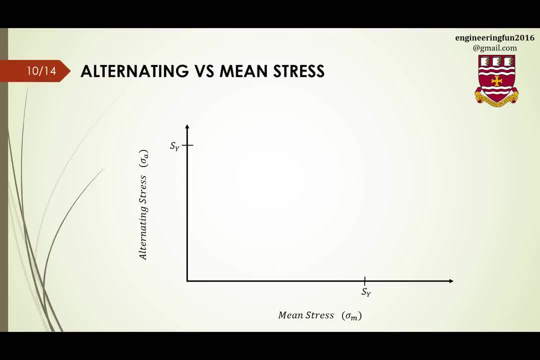 When mean stress is zero. Okay, I'm going to show like we are studying this one: This is sigma M and this is sigma A. When mean stress is zero, it means that we don't have any offset, So we are oscillating around the x-axis. 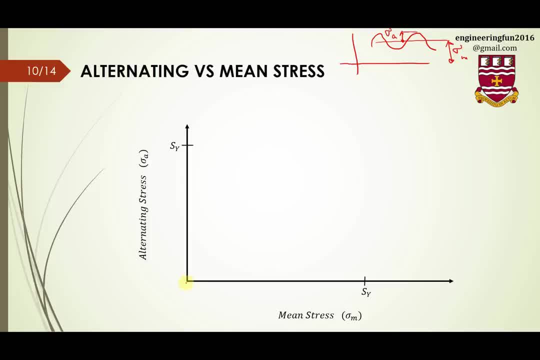 Okay. So when we are here, okay. before I want to: okay. So that's a completely reverse scenario. When alternating stress is zero, that means we don't have any amplitude. So that's the static type of loading. There is no fluctuation. 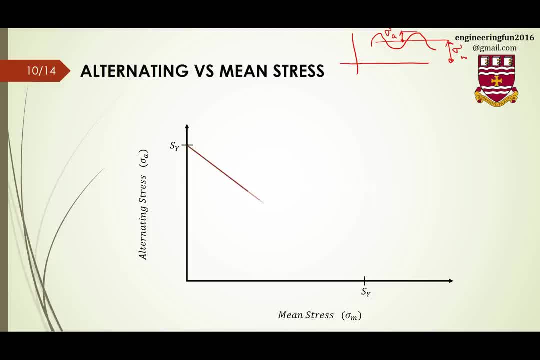 Okay, So yield strength is one of the important for us point. for us, If we draw a line between the yield strength in both axis, we're going to end up with a line and this is called Langer line or yield line, And based on each line, 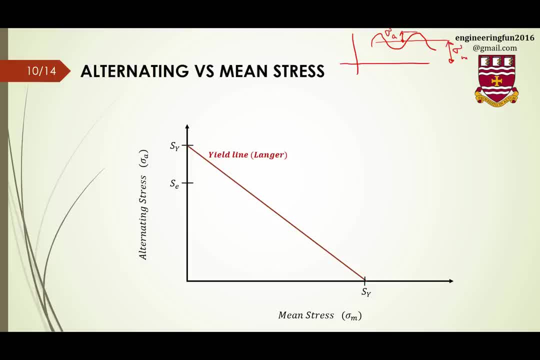 we define a scenario and based on each scenario we define or we find a factor of safety. So this is interest and strength. if we draw a line between interest strength and yield strength, this line will be called Soderbergh line And we can have different type of scenarios here. 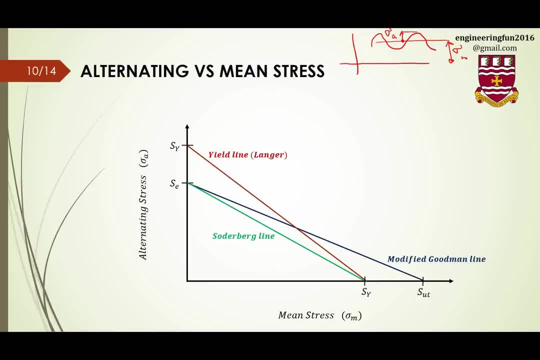 When mean stress is zero. so we said that we are in a completely reverse scenario. This interest strength is more important for us. This is what we discuss about that So far. we discussed about Marion equation- how to find this number. So this scenario. 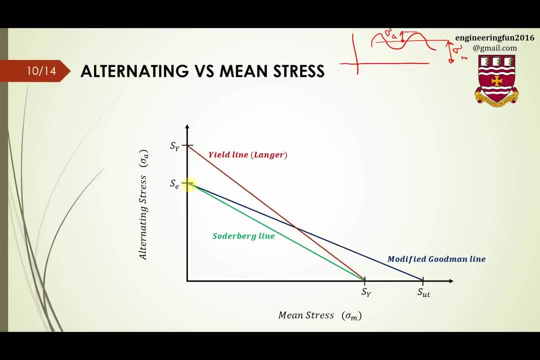 these scenarios that are starting from this point is somehow more conservative and better than considering Sy as our failure point. Okay, And when alternating stress is zero here, okay, we can decide. we can use Sy because that's a static type of loading. 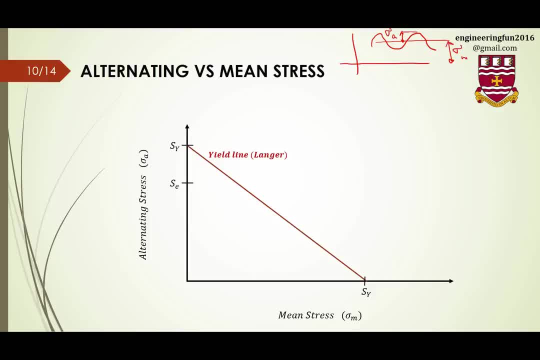 So if we come back to the, to my example I had amount of force was changing from 18 to 68. I'm say that area is 10.. Okay, So I can find maximum stress by dividing maximum loading over time, So that will be 6.8.. 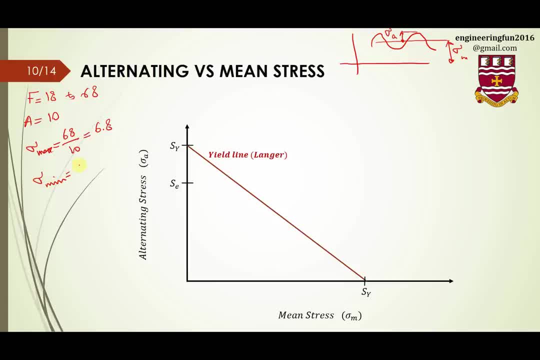 I can find minimum stress by dividing the minimum force over time. So that will be one over, one over. Both of them were tension force. If one of them was compression, we had to consider minus here. That was an agreement When we are in compressed. 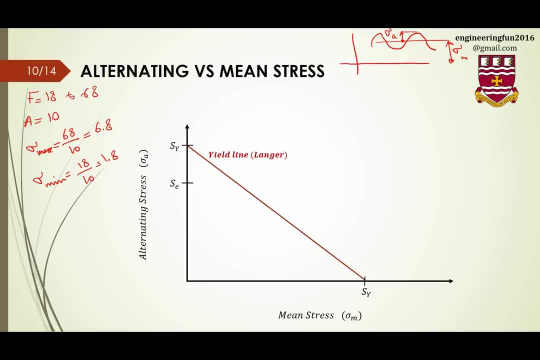 when we are compressed, the amount of stress is presented with negative, And when we are in, when we are stretched, we are positive. Okay, So this is minimum, maximum. I'm going to find average stress, which is the average between these two. 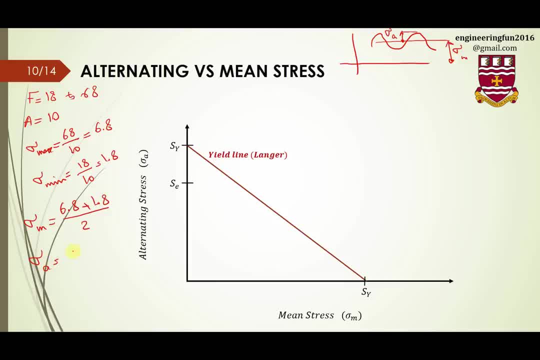 And I'm going to find alternating stress which is absolute value of these two. This is easier. That will be 2.5.. Okay, Yeah, it's 2.5.. And here that will be. so it will be 6,. 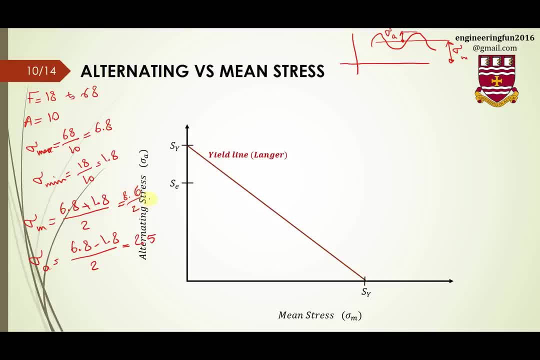 8.6 over 2, 4.3.. Let me double check. That will be. that will be 5 over 2, 2.5.. That will be 8 over yeah, 4.3. Okay. 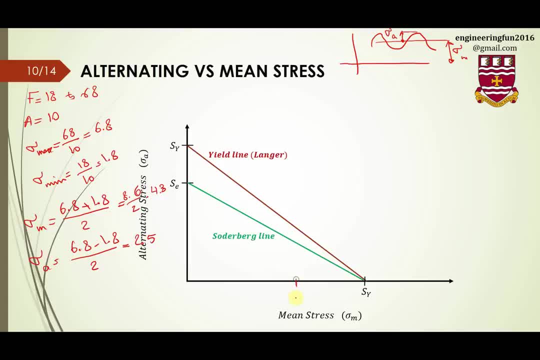 So sigma m is 4.3. For example, this is 4.3. And sigma a is 2.5. So this is 2.5.. In this case- oops, this is 2.5. And this is my point. 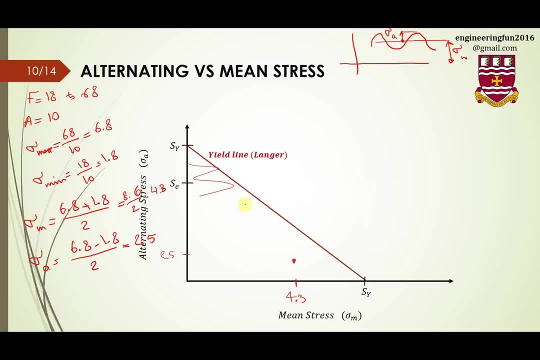 my load point. If I am inside this region, that means that I'm in the safe region, So I'm okay. If my point was something here, that means that I'm not okay. Okay, I'm going to talk about that one later. 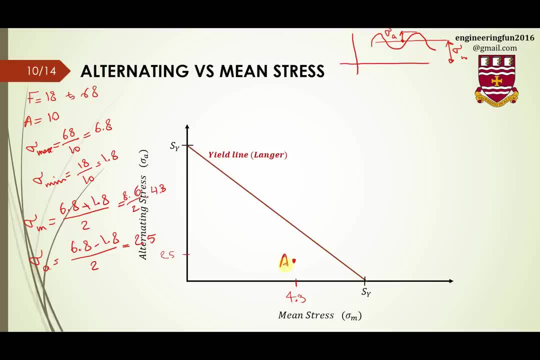 But let's say this is one point, point A For different type of question. we are here point B and point C, So we know that point C is not. okay, We will not talk about this one. Point A and point B. 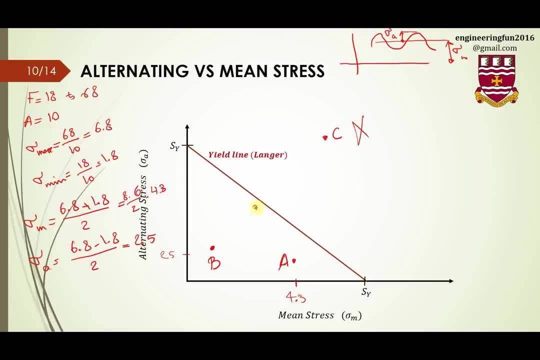 Which one do you think it's better? And this is point D. Maybe that's easier to discuss between point D and point B. Do you think point B is better or point D? Point B is better for us because this line is like an edge. 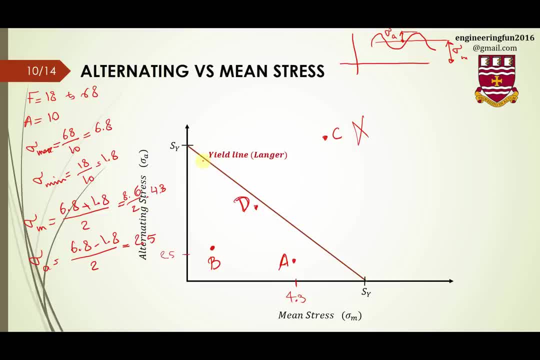 We are walking around the edge here. It's true that we are studying, we are studying around the edge, by the edge, but we don't want to walk around the edge. So the far we are from the edge, the better we are. 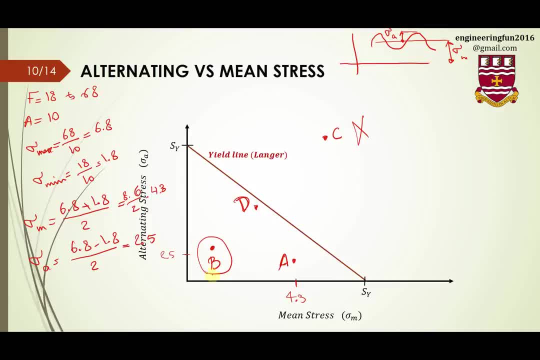 So this point is better, So it should have a better factor of say: oh, I'm going to talk about that later, Don't want to confuse you. Okay, That's the first thing If I want to compare these two points. 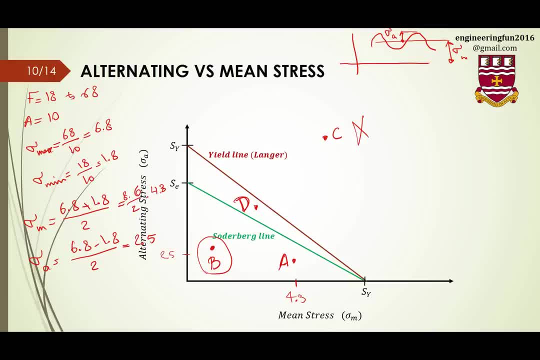 point D: based on Langer criteria, it's a safe point, but based on Soderbergh, it's not safe because it's out of the region. Okay, So Soderbergh is very conservative in comparison with Langer line. 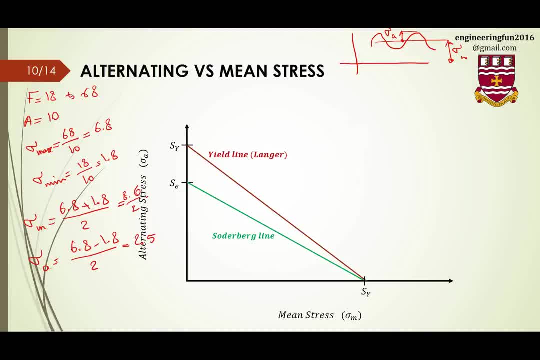 Okay, I'm going to remove these ones. Okay, Modified Goodman is not exactly the area between area covered by this line, this triangle. It starts from this point entrance to the intersection of Langer and Goodman line, Then it follows the Langer. 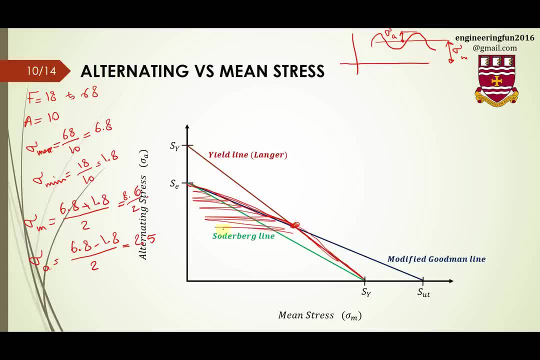 So this area is modified Goodman, So we modify Goodman and we found this area. So, for example, my point is here, based on modified Goodman. It's not in the safe region, So we have to be here, Okay, So don't confuse with this title here. 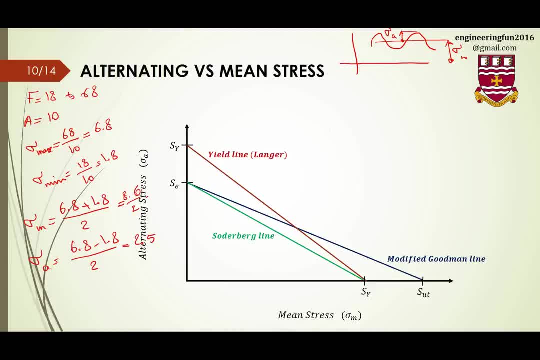 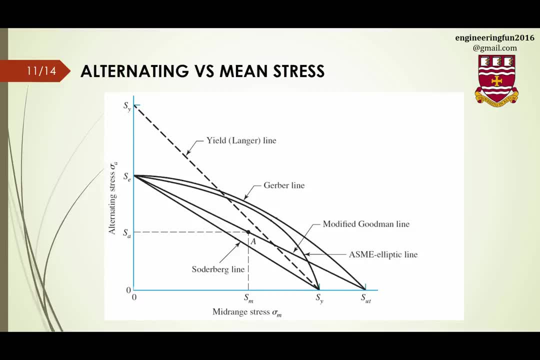 I should have put that one somewhere, maybe. Anyways, And these are the other criteria: Gerber line and ASME elliptic line. So ASME, this line, as it is shown in the name, it's an elliptic equation. 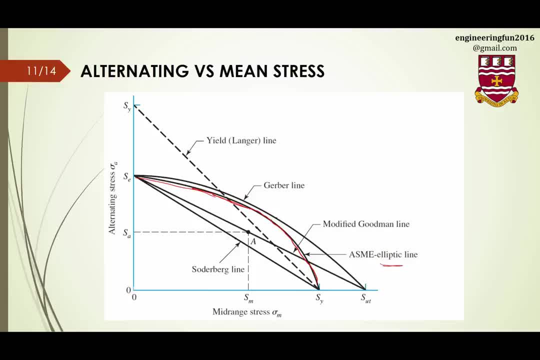 And Gerber line is a second order equation, a probability equation. This is the other one, And these two criteria are very good. if you want to use your design based on these two, I suggest you to do that in real life, But the problem is finding equations for these two. 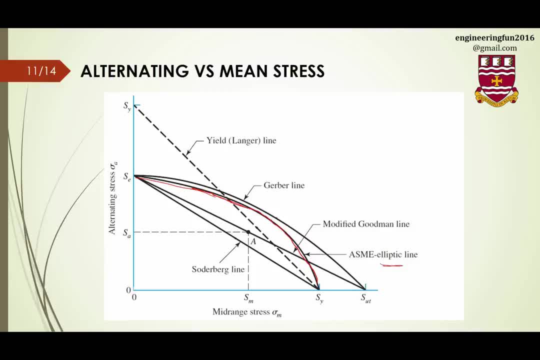 are very difficult, So maybe it's not a good idea to explain it here. But anyways, the problem with these two are it's difficult to find the equations, but they are very good criteria to use. So if this is our point, point A: 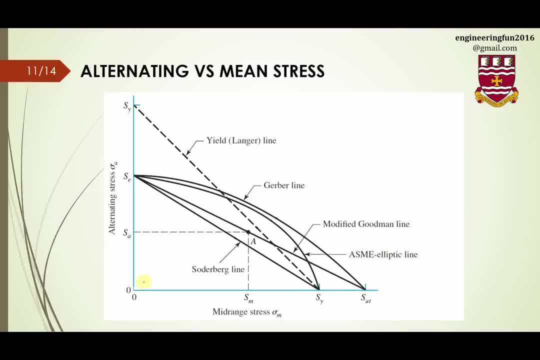 load point. we can draw a straight line between origin and the point And that line is called load line. So this is load line. Okay, So slope for the load line. if that's my load line, this is rise. is rise over run. 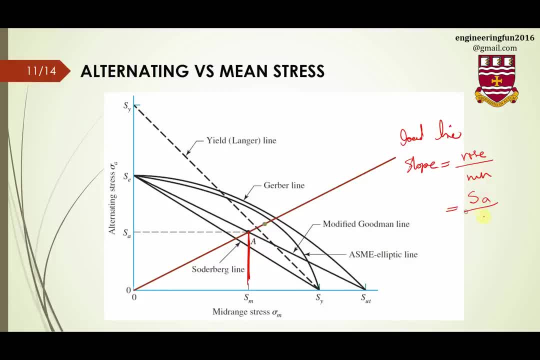 Rise is SA, Run is SM, This is theta. here I better say: slope is slope, is tan of theta, And tan of theta is rise over run And this is the slope. Okay, If my case was not this point A, this point A is not a good point for. 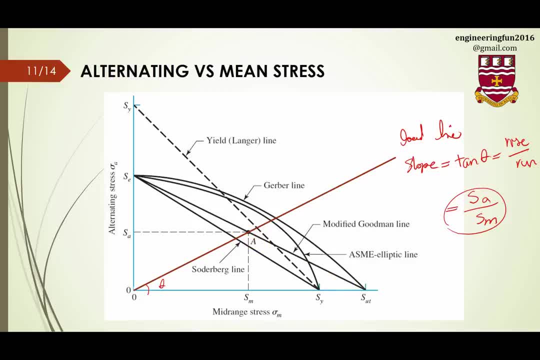 presenting at this slide, because the intersection between this point and this line is occurred on the line, on the load line. If I have a load line like this. these are the important points for me: The intersections of the load line and each criteria. 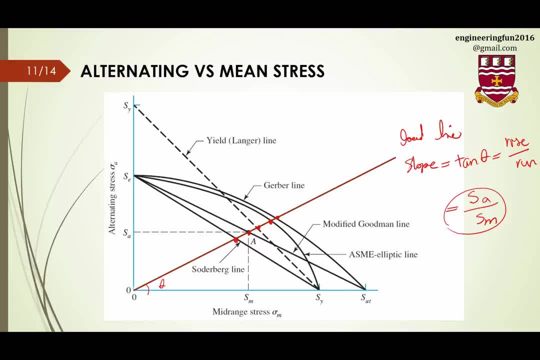 Because we're going to define some safety factors, some graphical safety factors, based on the distances. these distances: Okay, If my point line was this, green point here, Okay, So there is no intersect between this point and any of these criteria. If I draw a line, 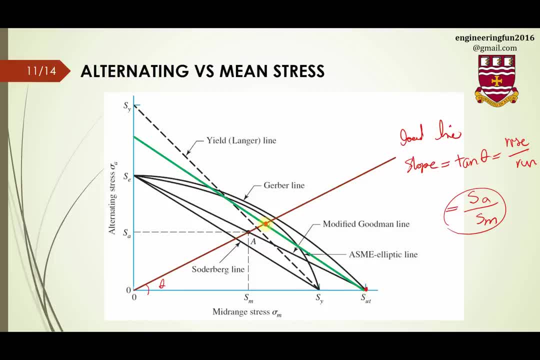 from SUT passing our load point. the intersect between that's load, that's line- It's not called load line, That's line- And alternating stress is going to give us reverse stress And that's a completely reverse stress If you want to find completely reverse stress. 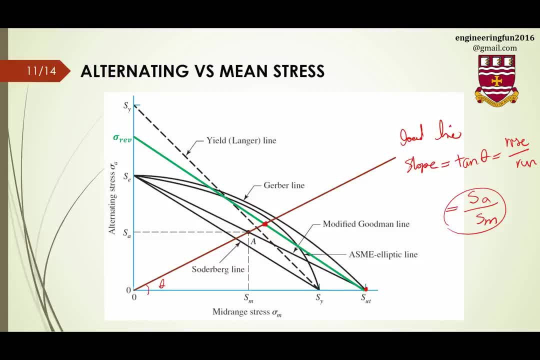 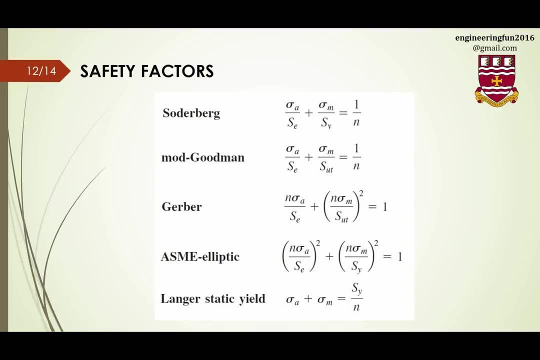 based on a diagram which you are asked in your question, your problem, your tutorial problem last week. you need to draw a line here and you need to report this number. Okay, Safety factors. Based on each scenario, we're going to have one equation. 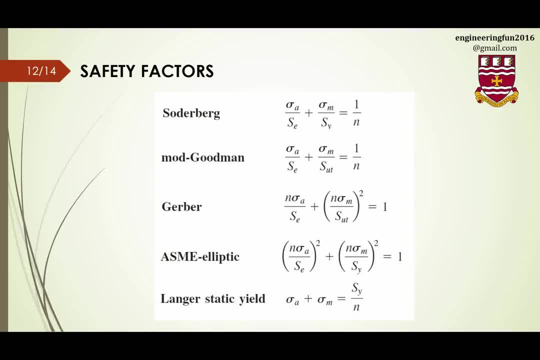 For example, if you want to find safety factors based on Soderbergh, this is safety factor. We have sigma A, sigma M. we have indriance strength and S-Y yield strength. we can find N If we want to use ASME elliptic. 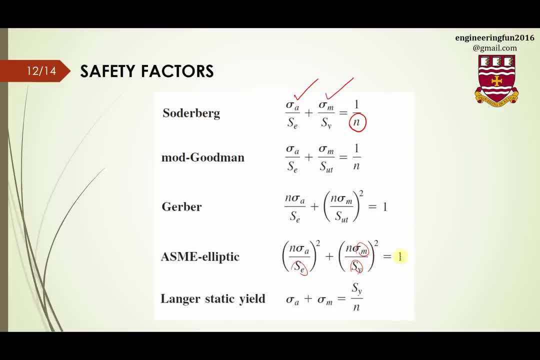 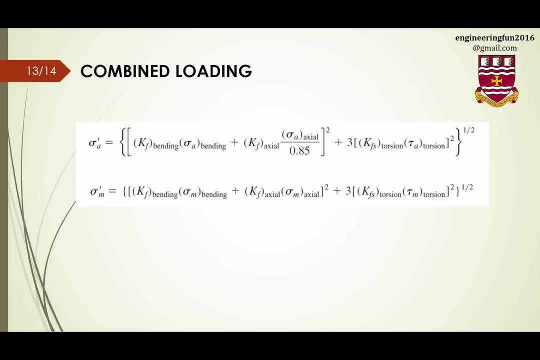 we know sigma M, we know this one, this one, everything but N. So N can be found from each of these scenarios. Okay, Sometimes we have a combination of loading on a specimen. In those cases, instead of finding sigma A and sigma M, 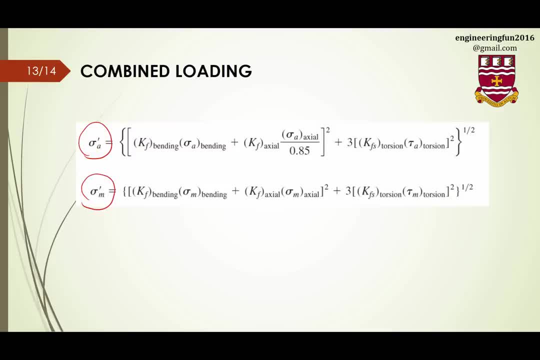 we need to define sigma A' and sigma M' In order to find that you can use these two equations. And there are some factors And when you multiply those factors by the type of loading that you have, you're going to find an equivalent. 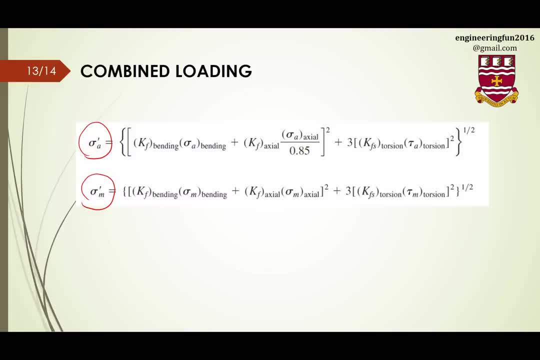 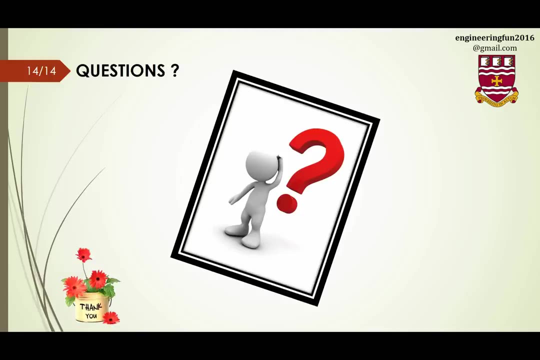 sigma A, alternating and midrange stresses, And then you can just use that one and plot your sigma A' sigma M' and do what we did for the previous step. Okay, If you have any questions, feel free to comment below Before I want to finish this one. 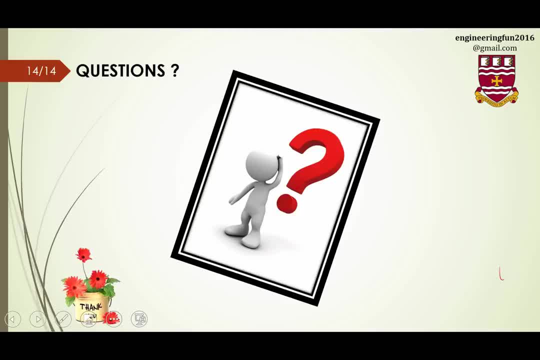 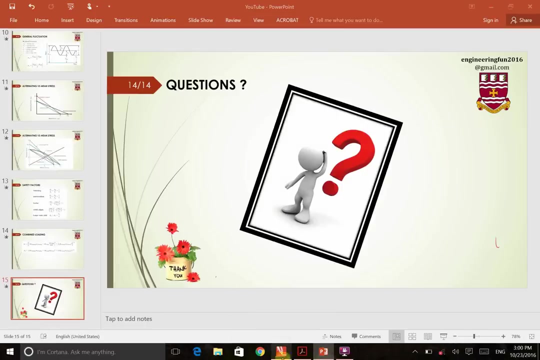 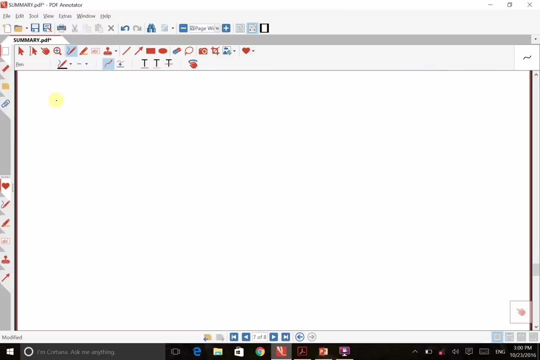 I'm gonna review, I'm gonna have a quick review about what we covered in these slides. Okay, Yeah, skip them, why not? Okay, We said that everything starts from internet, from online or from table A20.. And again, 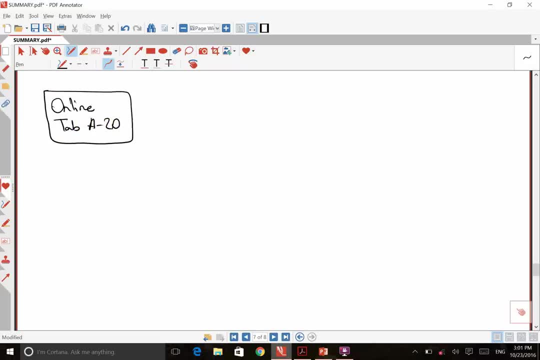 I'm saying that all the tables and graphs that I'm gonna mention now is based on 10th edition of Shigley's book, And if you haven't bought that, maybe it's a good idea for you to pause the video and find the book. 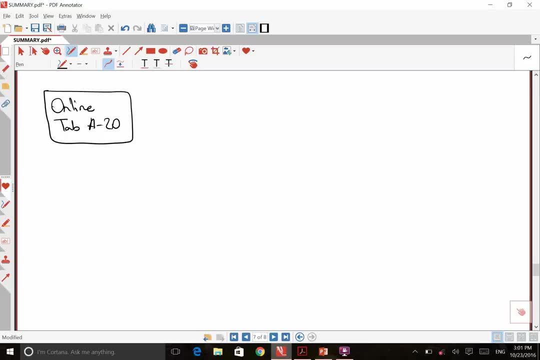 Find the book somewhere online or order it from a website and get the textbook Okay. from this table, what we can read is ultimate strength or yield strength. For some materials, yield strength at tension and compression are different, But these are the material like. 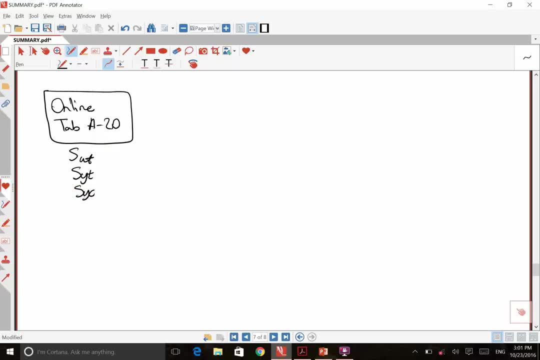 properties that we can find from. This is for steel, I believe Maybe a steel 1820 or 1810. But we can find those prime conditions. We can find those parameters. When we find that one, we need to find S E prime. 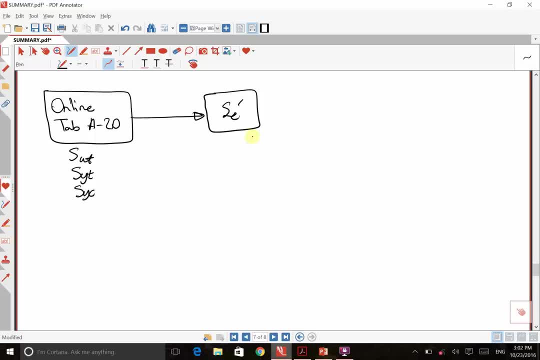 S E prime is endurance strength for a, for an ideal specimen. In order to find that one, you can use equation 6-8.. So equation 6-8.. Maybe I can write it here, The equation 6.. Equation 6-8. 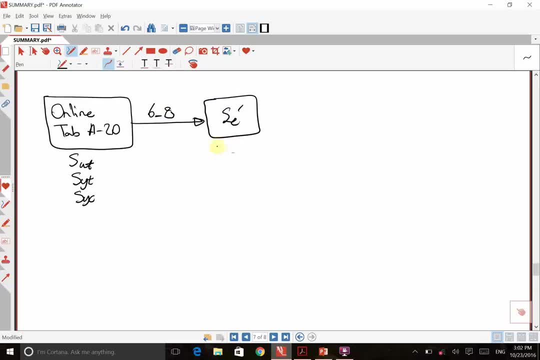 is related S E prime based on that. So S E prime is a function of S U T Okay. So when you get S E prime, you need to find endurance strength, And here you need to use equation 6-8.. 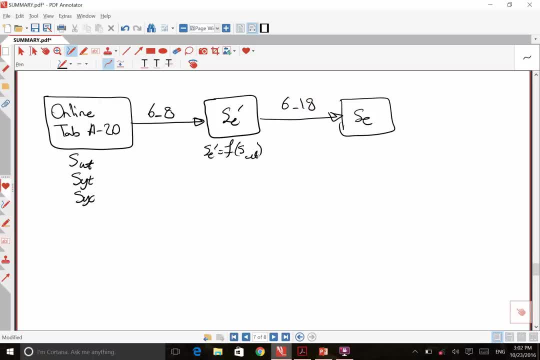 And So S E is a function of S E prime, And these are: This equation is called a marine equation And we have a couple of factors here. Okay, We have K? A that can be found from equation 6-19.. 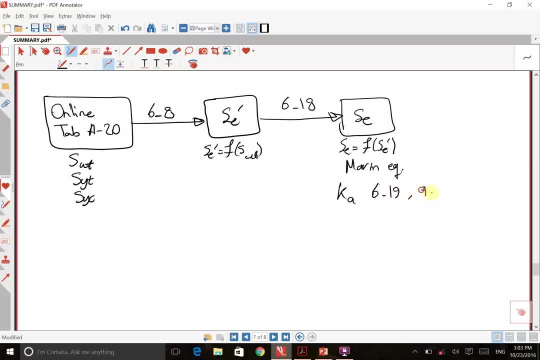 And table 6-2.. We have K B that can be found from equation 6-20. And 6-21. And table 6-3.. We have K C that can be found from equation 6-26.. 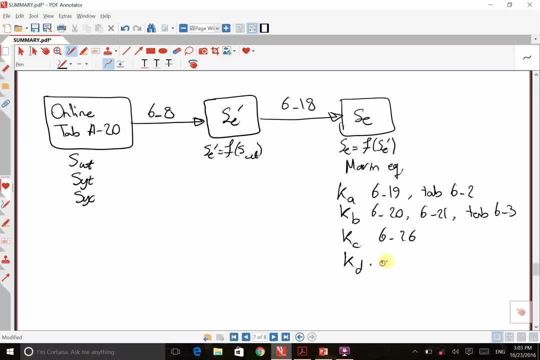 We have K D that can be found from equation 6-27.. We have K E, that can be found from table 6-5.. And K F, which is other factors, which is for other factors. Okay, So when we get this S E. 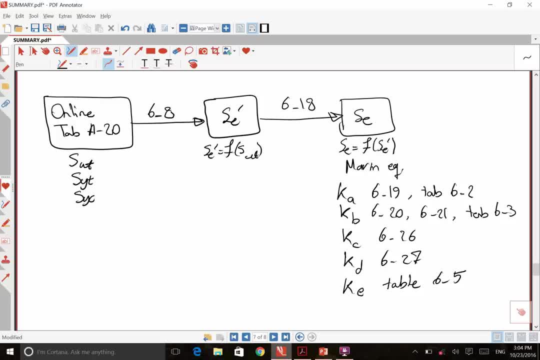 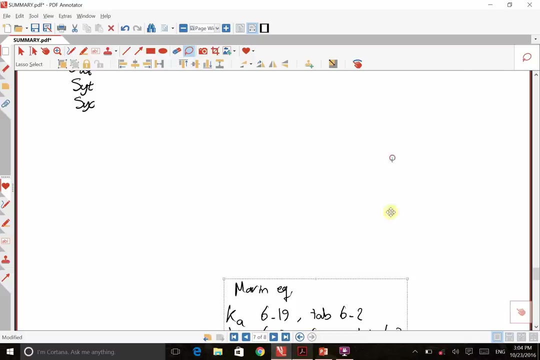 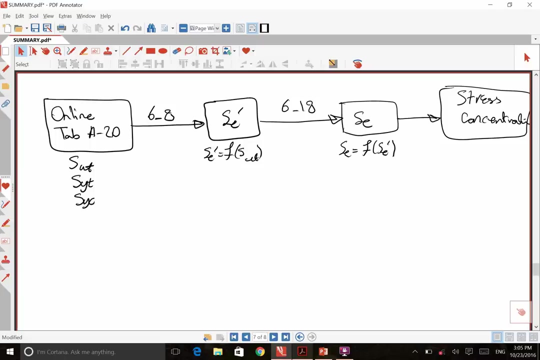 based on marine equations. so these are marine factors. we're going to check something here, I don't know. We're going to check stress concentration. Okay, Let me take these ones. Okay, We're going to check stress concentration If the material 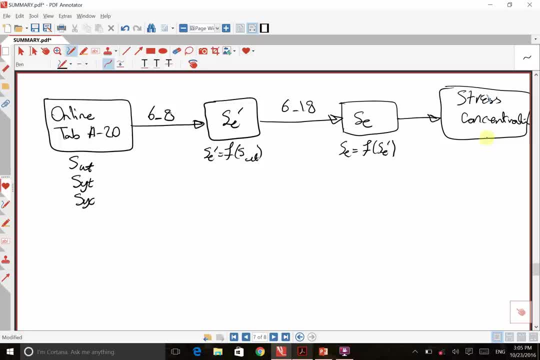 like If the material. there is no notch, no radius, no fillet, no hole in it. so we are in the no part. But sometimes, and I'd say most of the times, there are some stress concentration sources in the material. 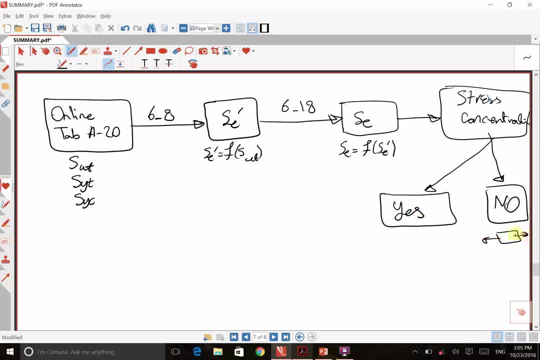 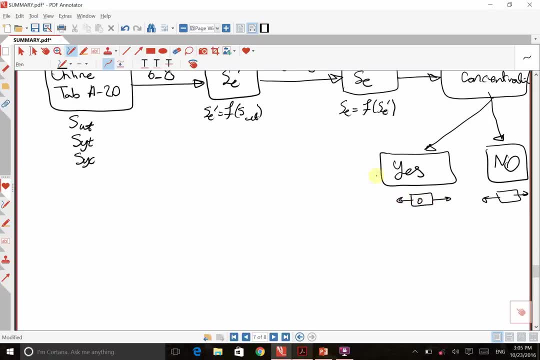 So this is, for example, this is for a material like this, and this is for a material: the stress concentration. If there is any stress concentration sources, we need to find K, T, That's capital K, Theoretical stress concentration. 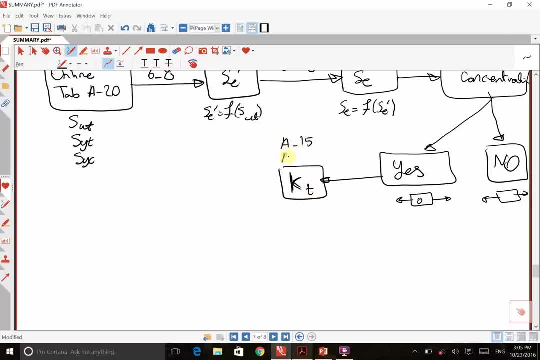 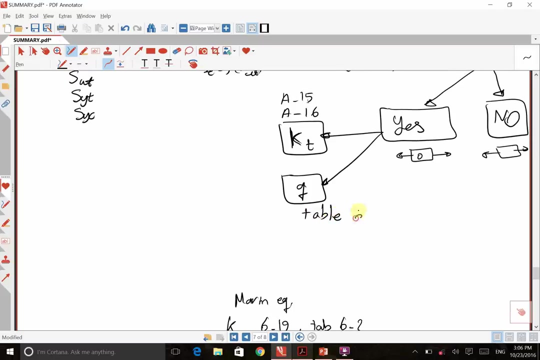 And this can be read from A15 and A16 appendix, table 15 and 16 appendix. And we need to find notch sensitivity Q And this can be found from from table 620 or 621.. And 621, or equations 634 and 635.. 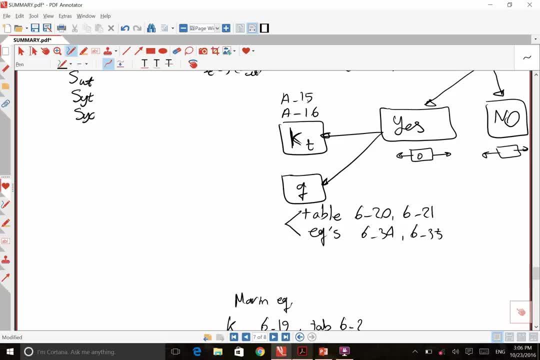 So there are two ways to find this: Q, You can use whatever you want, And once you get that, you're going to find K, F based on these two parameters. Okay, So if there is no stress concentration, we jump to this step. 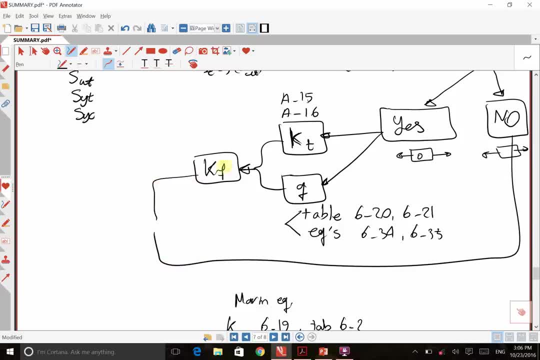 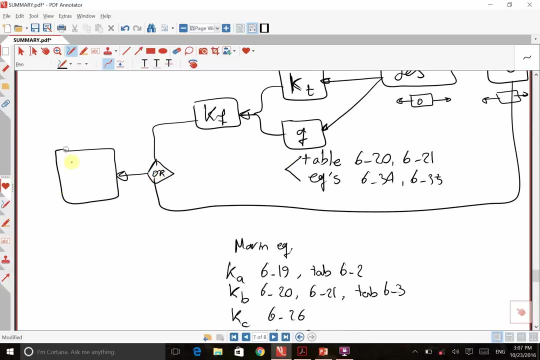 But if there is some stress concentration, we need to do these parts and find those. find K, F, Okay. So I'm going to say so after this point, we're going to find maximum and minimum stresses. Maximum is F max over the area. 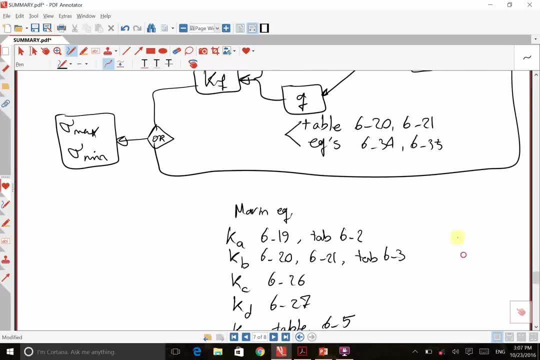 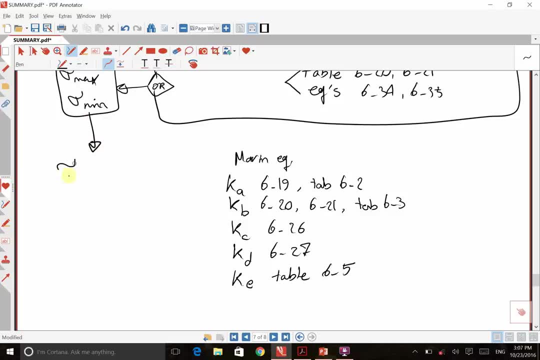 Minimum is F, min over the area- Area could be different in different questions And once we get these stresses, we're going to find mid-range or mean- oh sorry, mid-range- or average stress, which is sigma M and sigma A, And this is equation 636.. 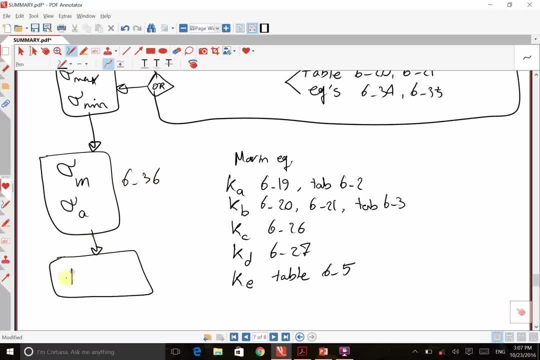 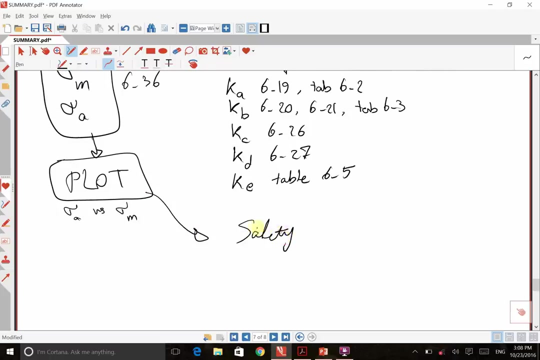 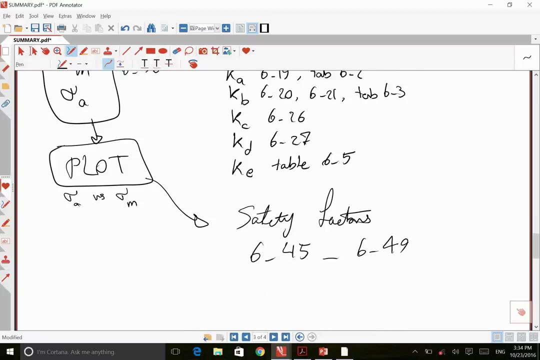 And when we find that one, it's done Plot. So we can plot sigma A versus sigma M, And if you're asked to find safety factors, safety factors can be derived from 645 to 649.. Okay, There is one thing here. 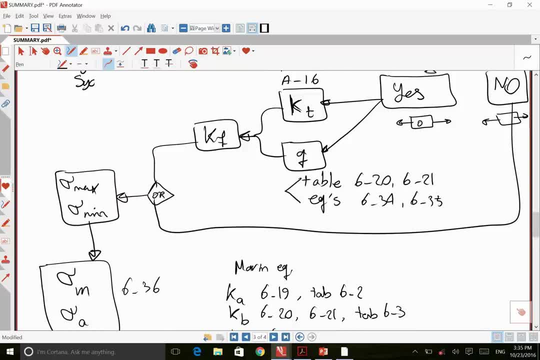 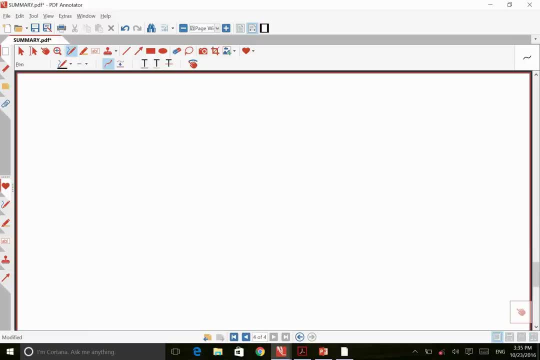 When you find this safety factor- fatigue, safety factor K F- we need to somehow use that And I'm going to mention, bring that one to your attention at this page. For example, if our mid-range stress can be found from this equation: 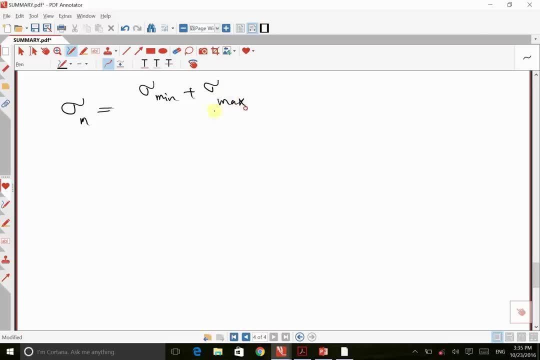 the average of mean and max stresses. this is for a specimen without any hole. If there is any hole or, for example, if there is something like fillet in the specimen like this is the fillet with the radius of R. we are going to find a safe. 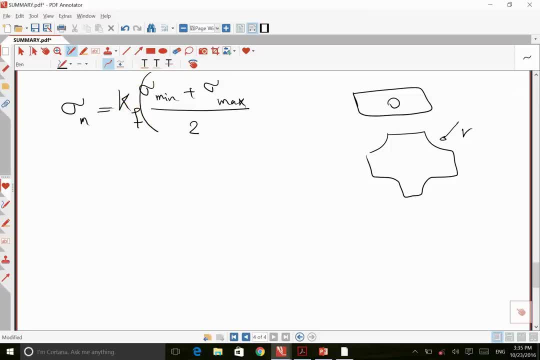 a fatigue safety factor- sorry, fatigue stress concentration- And we're going to multiply that one by the whole fraction, And the same thing happens for alternating stress. So that will be K F times maximum stress minus minimum stress, divided by two absolute value. 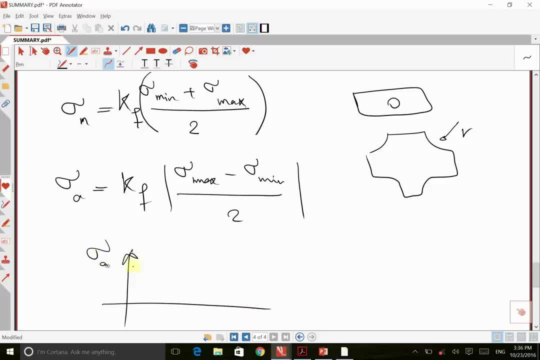 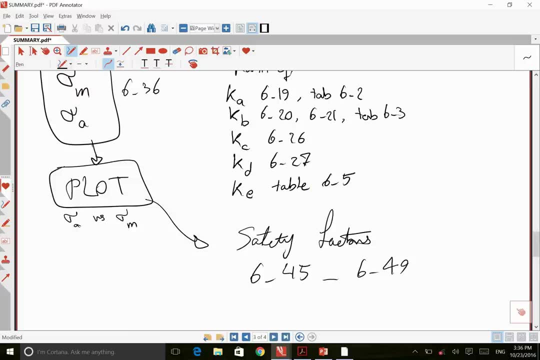 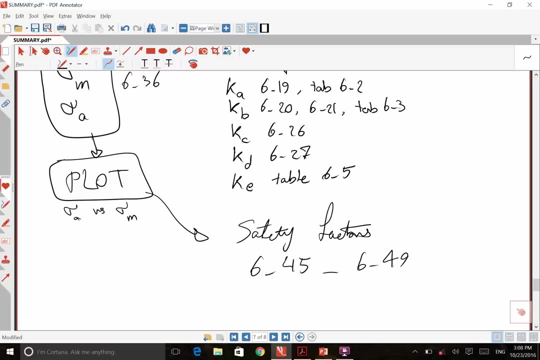 And we're going to plot sigma A over sigma M for these evaluated numbers. I think this chapter is covered, maybe 80% of this chapter, 90% of this chapter, And if you have any questions, feel free to ask. Send me an email at. 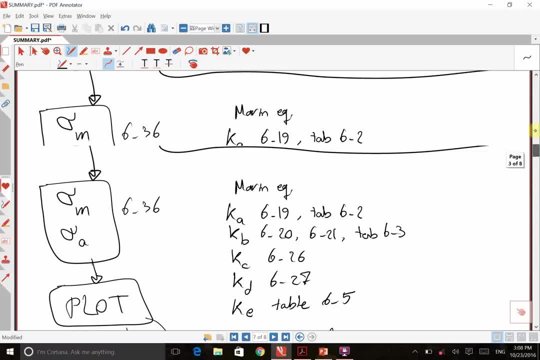 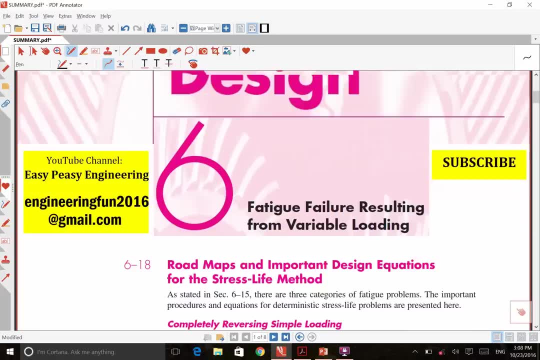 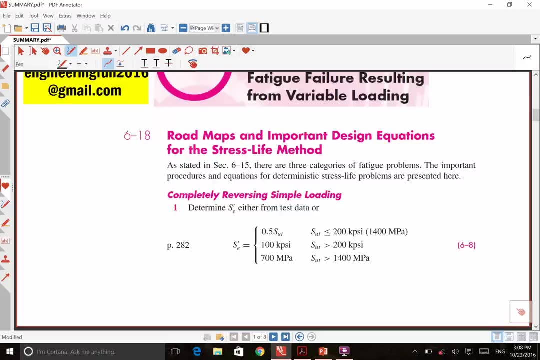 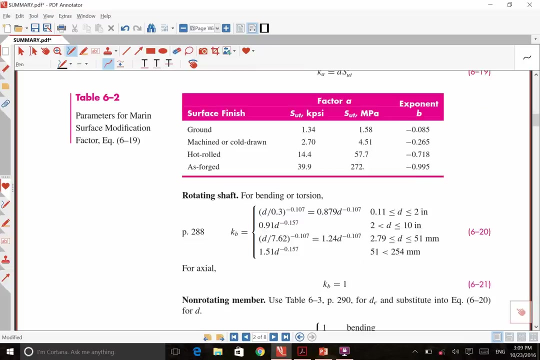 engineeringfund2016 at gmailcom and I'll be happy to answer them. Okay, So in part, this is a better review here. And S A, S, E: these marine factors are shown here in these notes: What is K H? What is K B? 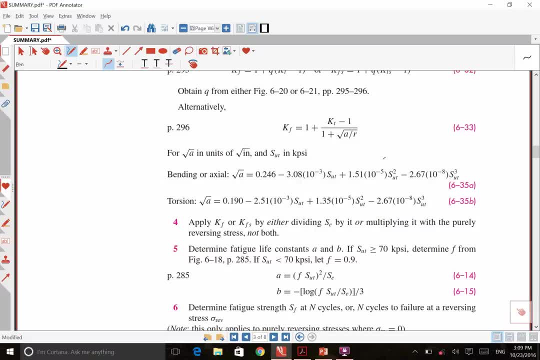 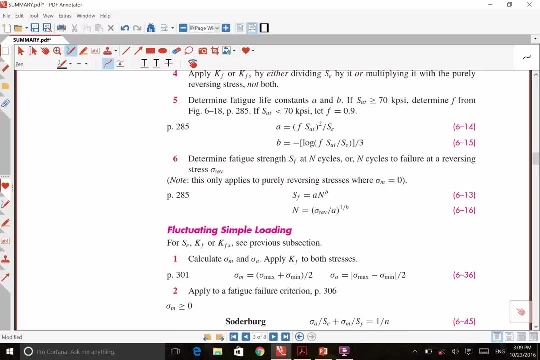 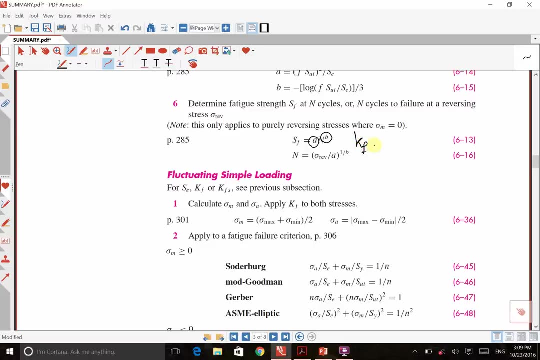 K C, K D. How you can find that? We talked about that. How you can find K F? What is square root of A? These equations, And we said that these A and B are different from A and B in K A. 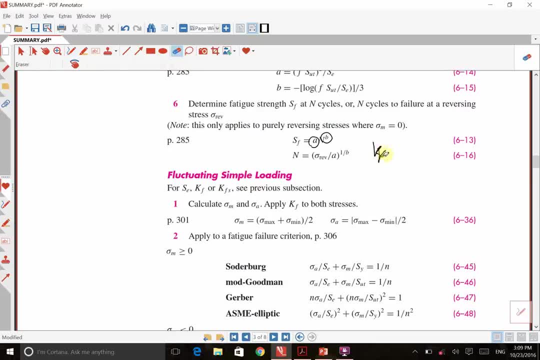 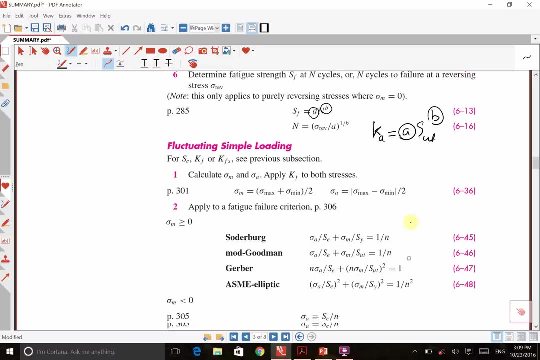 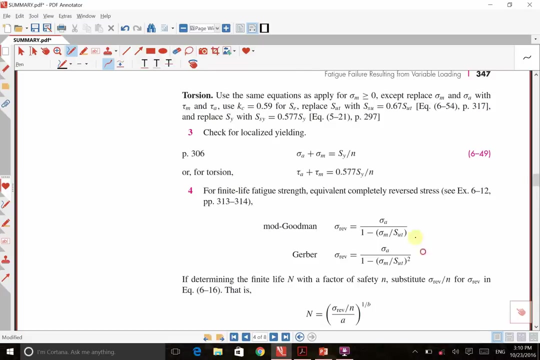 K. Okay, I think this pen is tired. K A is A S U T square root of D. These A and B are different from these two. These are found from a table based on material properties as safety factors for each scenarios, And yeah. 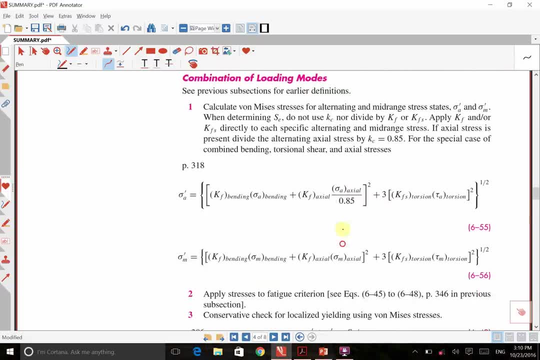 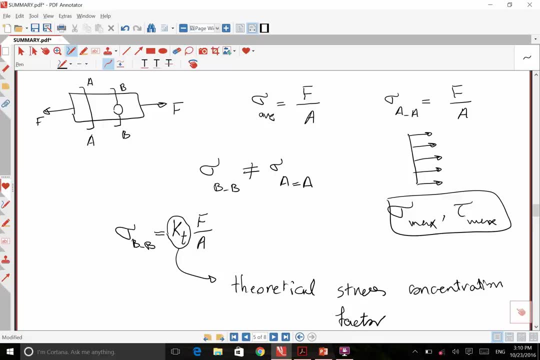 everything is almost covered in these notes and in this slide. I hope it can help you study this chapter better and I hope it can answer the questions that you had in your mind. Okay, Thank you for your time.